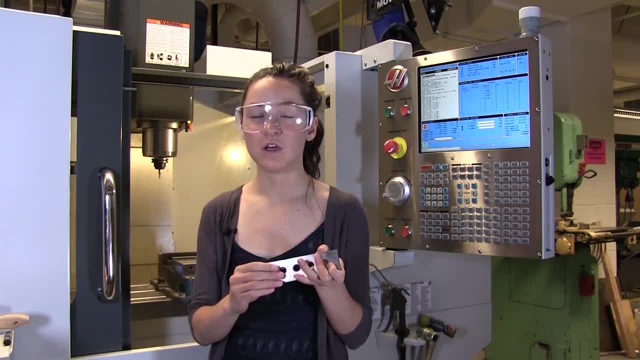 They're machined in sets so they're perfectly flat and square to each other. We're going to use these to help mount our stock in the vise. So before you put anything in the vise, you're going to want to make sure that everything. 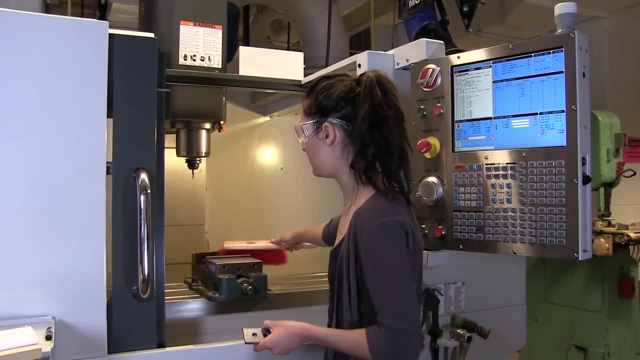 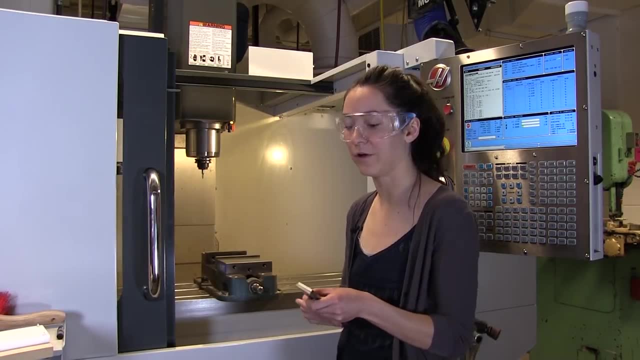 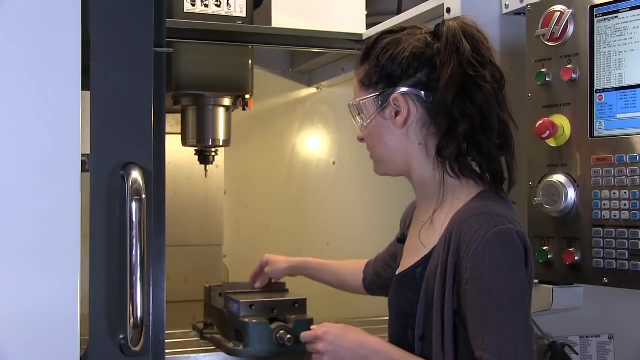 is in place. Before you put anything in the vise, you want to make sure that it's clear of any debris. This just ensures that you have a flat surface to mount your part on. So we're going to put these parallels up at either end of the vise. 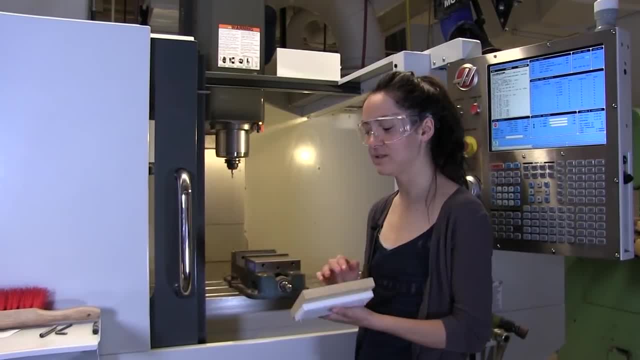 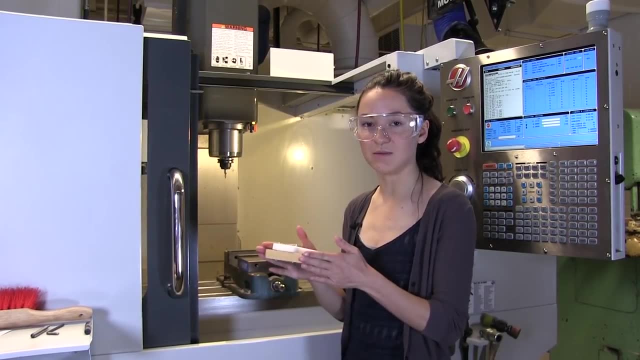 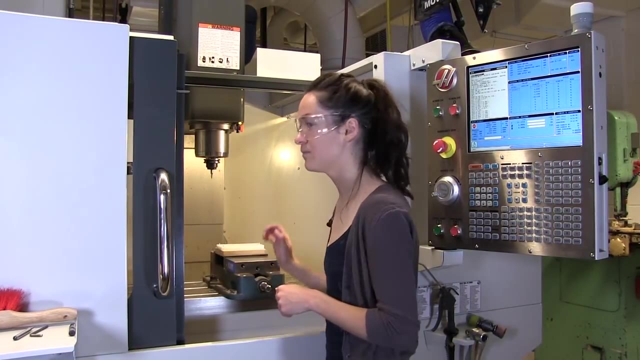 And then we're going to set our stock on the parallels. so the bottom edge is resting on top of these parallels And the edges are going to be on top of each other And that is going to give our stock break control Once we've set the workbite down, all of our stock in place, all the way through. and now. 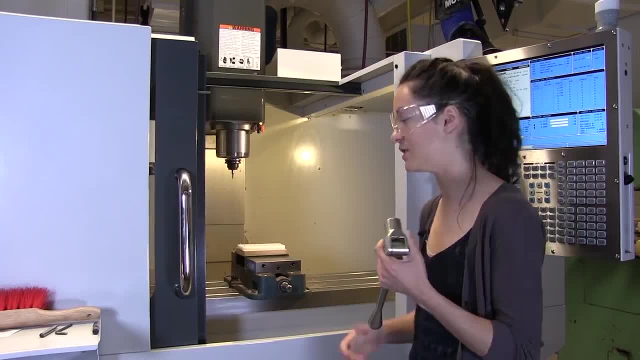 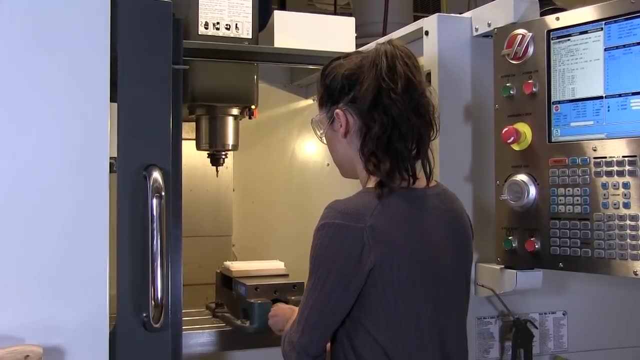 our finish stock is set up. I've removed everything that we. Section H is tangled up after Now, once we get our stock in place, I have the Der Terra nozzle put together And I have these relate when I tie the vise on here. 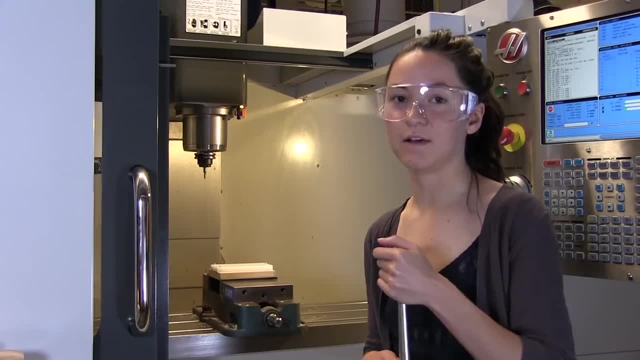 And then I get these súper tight holes. They're going to be twice as loose when it's tied together. Once they're in there like that, I'm going to use these handles here- that's just to the right on this rack- to tighten this down into the vise. 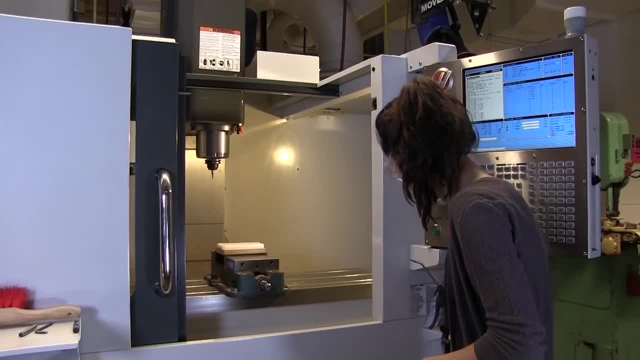 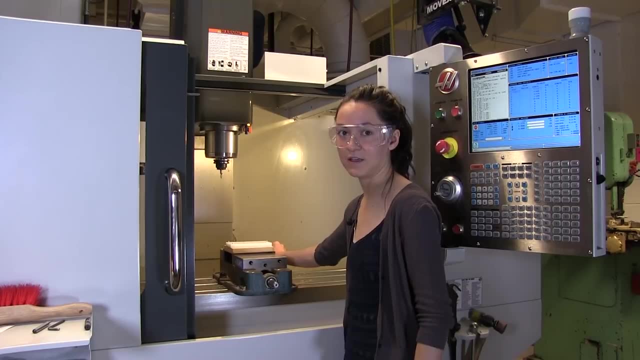 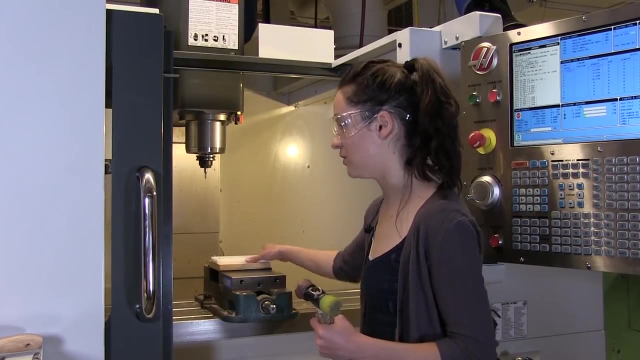 When we fasten these, I want to make sure that the quarter should be safe at the same time as you're ỹ racing through this to be overly tight. Next, I'm checking that these parallels are stuck underneath it. See how they can move. We're going to use this rubber mallet to hammer down the stock, so 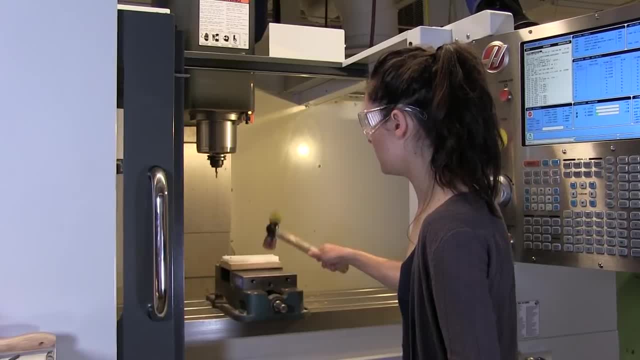 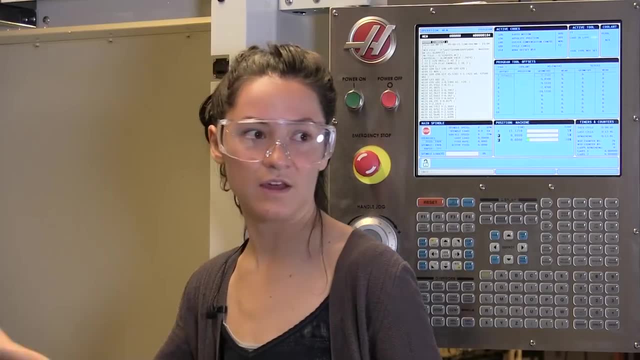 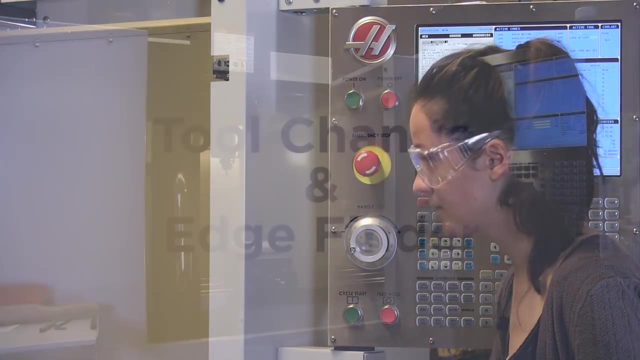 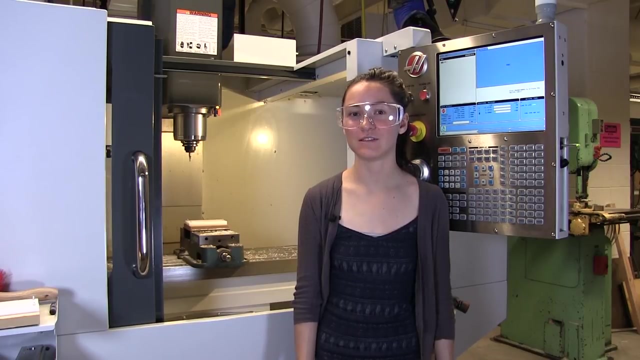 that those parallels can't move underneath it. Now that they're not moving, that ensures that the stock is completely flat in the vise. now, Now that your stock is in the machine, you're going to have to tell the machine where the stock is located. To do that, I use the 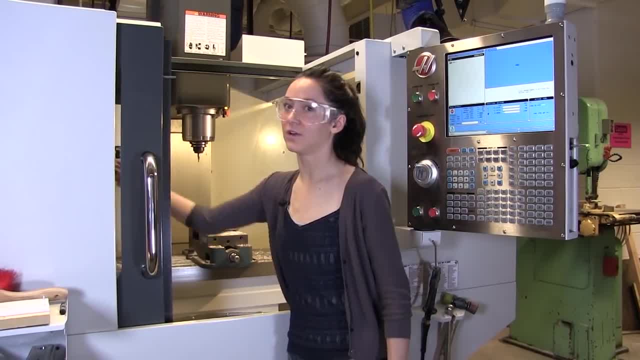 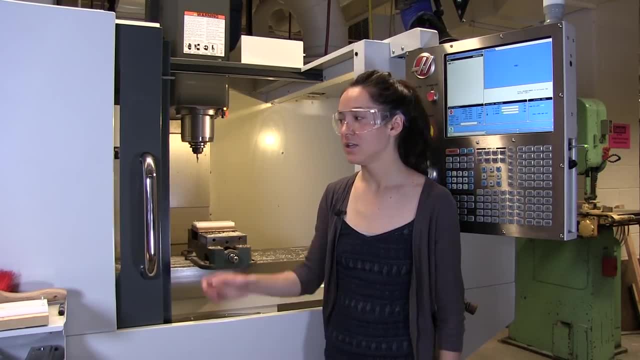 edge finder tool which is located in tools. This is tool 4 over here. I want to bring it up into the spindle so I can use that. To do that. I need to do an automatic tool change. The door of the machine needs to be. 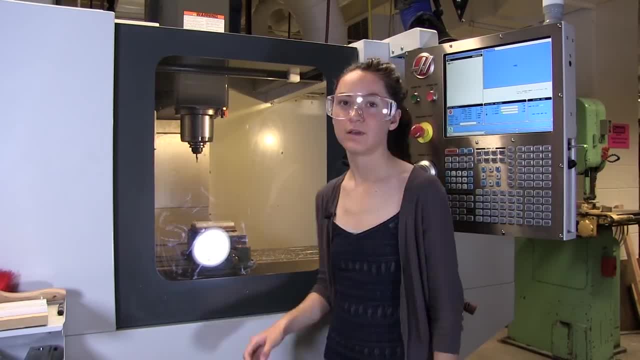 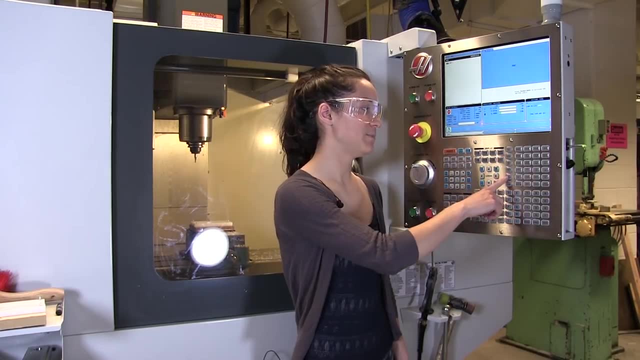 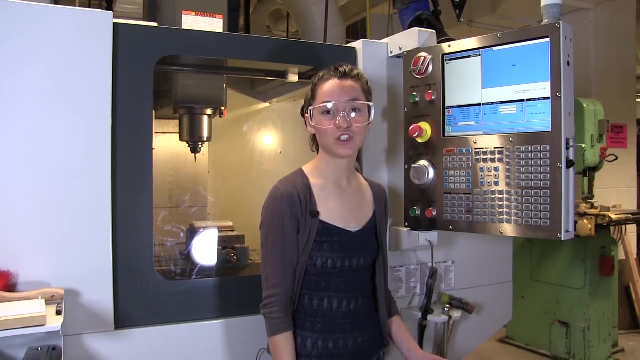 closed for it to do this, Then I'm going to get into the correct mode or menu to move this over. These buttons here I call mode or menu buttons. That'll get you into the correct mode in order to do tool changes or to move the table around. 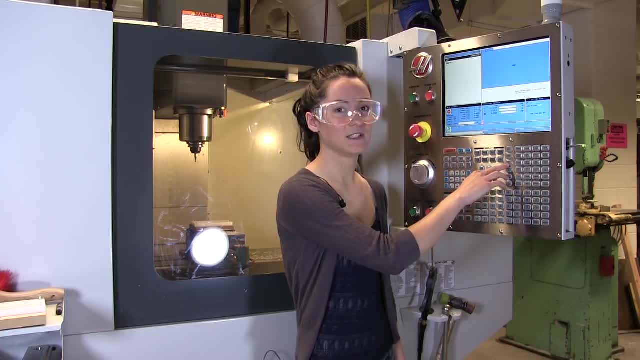 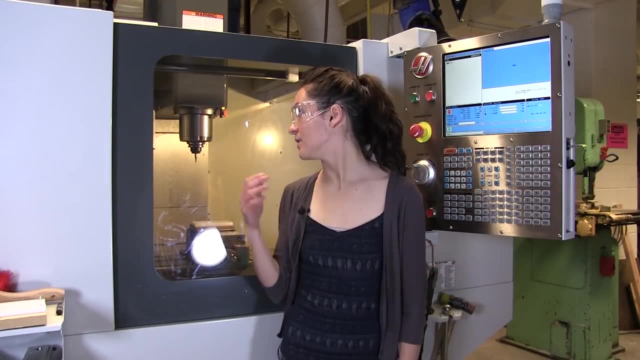 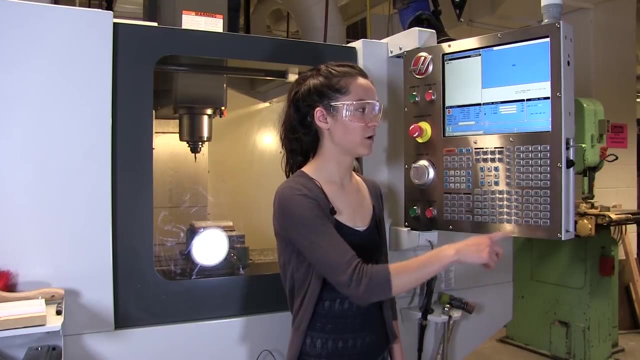 This MDI DNC button- MDI stands for manual data input- will get you into the correct mode to move the tool, Because it's several tools away from where we're located. now I'm going to type in the tool number T for tool 4 for the fourth slot. After you do this, 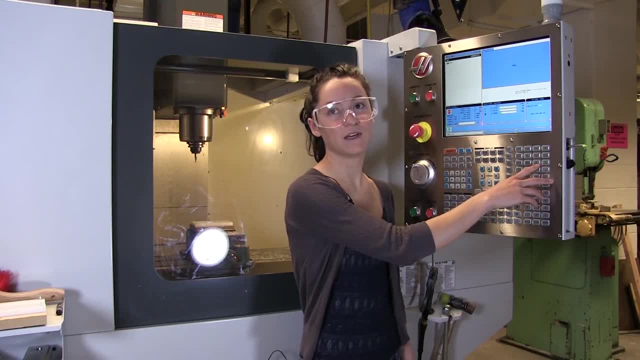 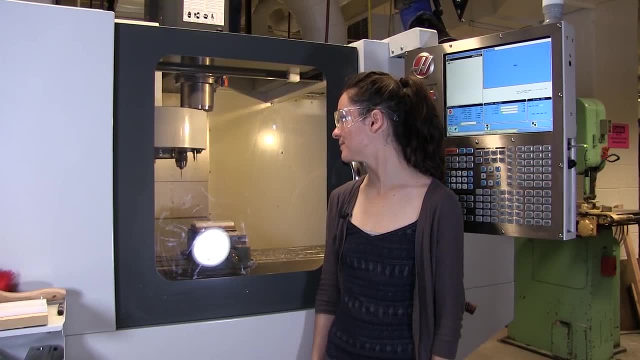 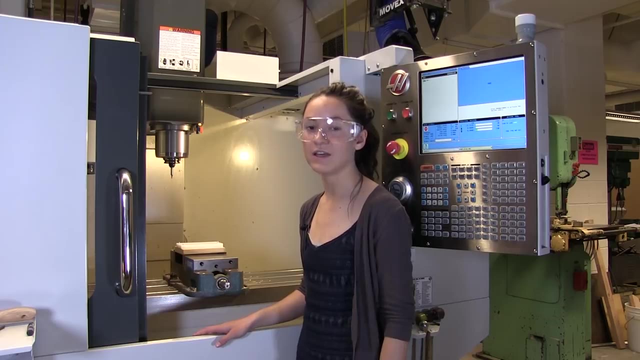 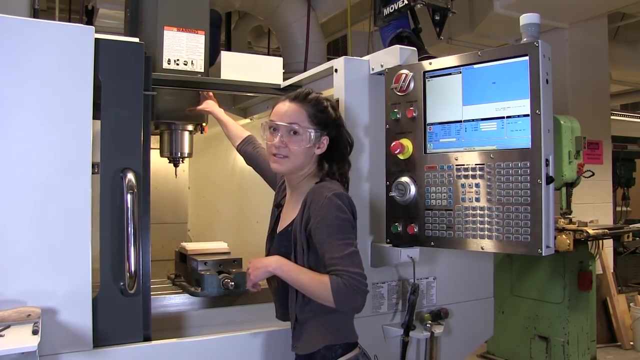 you press ATC forward or reverse will do the same thing. ATC stands for automatic tool change. All right, so now the edge finder is in the tool slot. I'm going to show you really quickly how to take the tool in and out. There's a button right behind this that you press to. 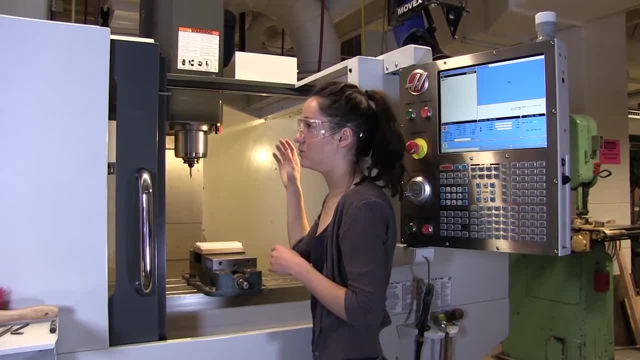 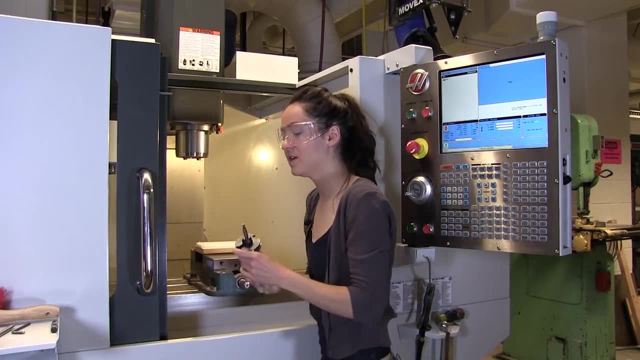 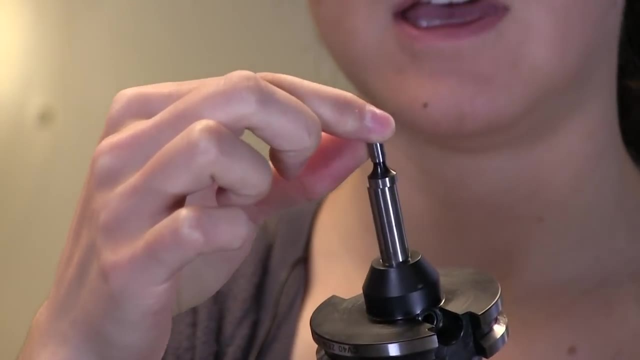 release the tool. When you press it, the tool will drop out of the spindle, so make sure you're holding onto it. This here is the edge finder tool. see how the tip of this can move back and forth. how this works is it's going to be in the spindle. 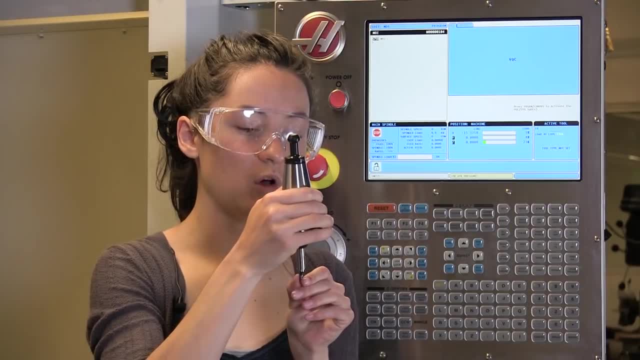 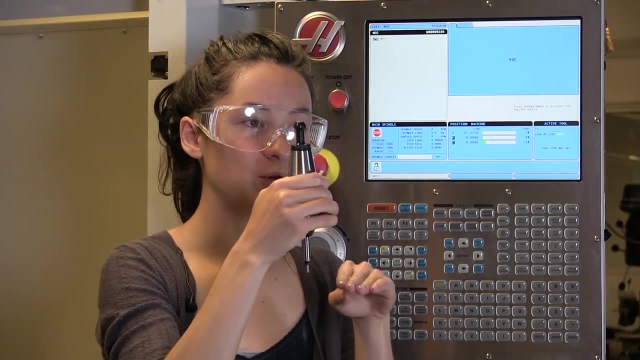 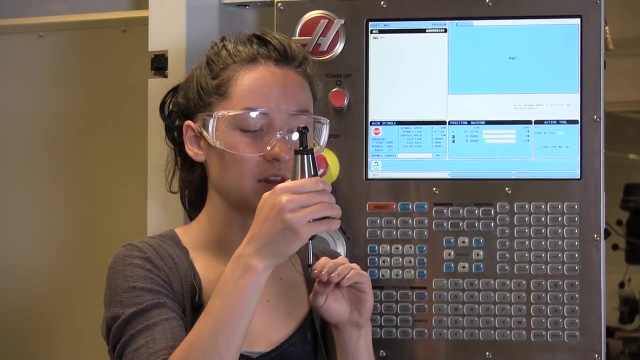 it'll be rotating and this will be wobbling around. you're going to bring your stock in close until it hits this edge finder and then it'll push it to go concentric with itself and it won't be wobbling anymore. at this point you're going to go really slowly and bring the stock in even closer. 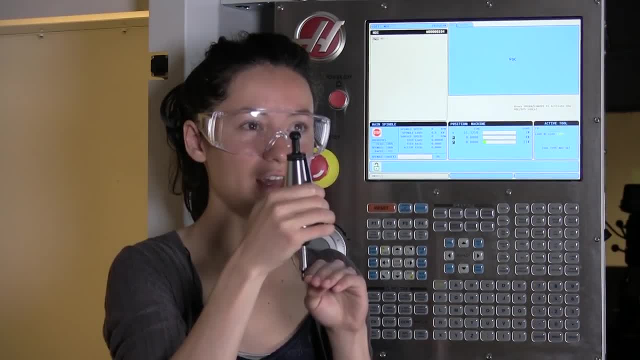 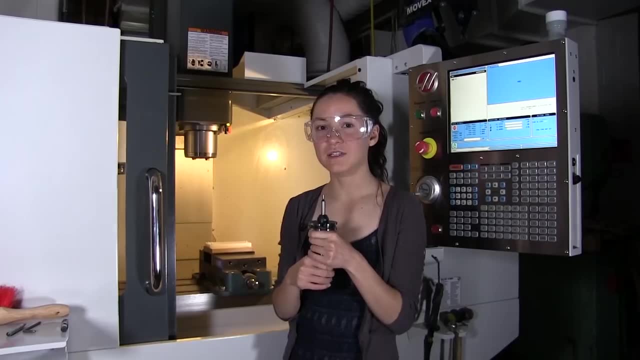 until it bumps off to the right. that's when you have found the edge of your stock relative to the edge of this tool. you need to tell the machine where the center of this tool is over the edge of the stock, because that will be the center of every tool in the machine. 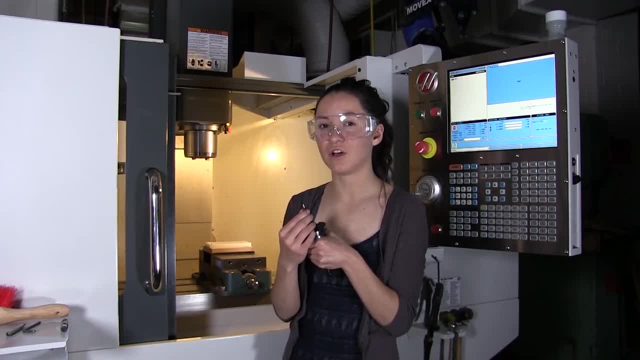 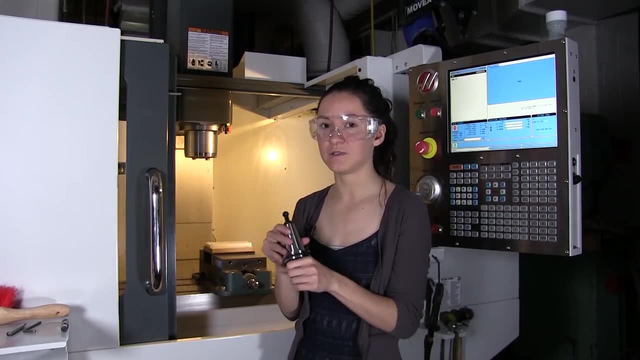 relative to the edge of the stock. to do this, you have to compensate for the radius of the tool, which is 0.1 inches. and i'll show you, guys, an easy way to do that. first you have to put the tool back into the machine, and then you're going to pull it out of the machine, and then you're going to 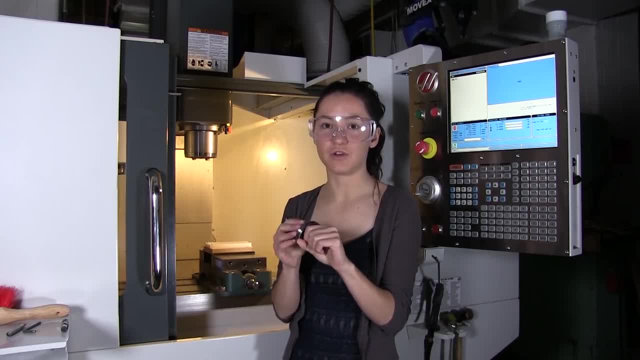 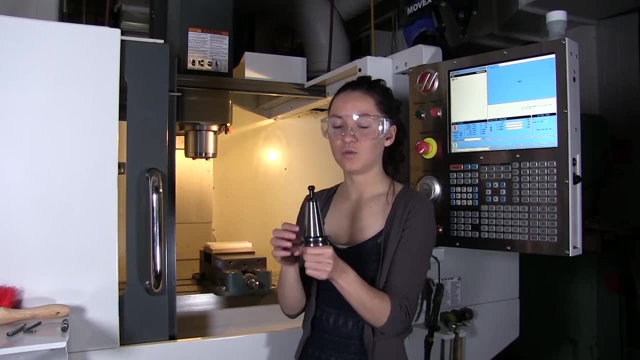 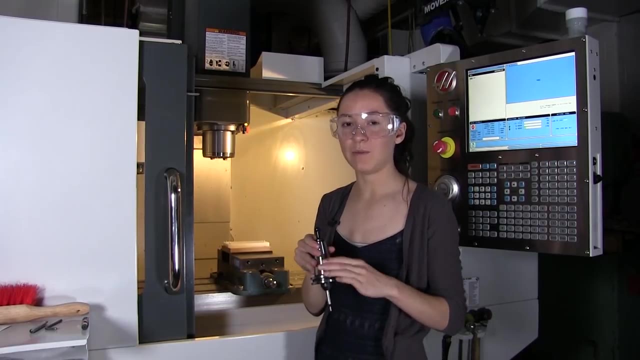 hold it just like this sort of like an ice cream cone. some tools have more to hang on to, but in this case you can just rest it on your hand. you're going to want to line these notches up with the pegs in the spindle. the machine will grab onto the tool even if you don't have those. 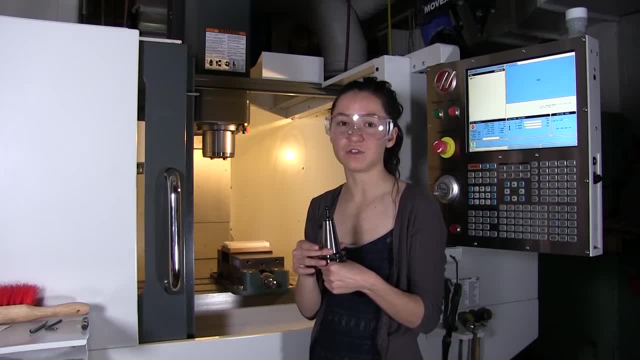 notches lined up, but you can risk throwing the tool if the spindle turns on, so you want to ensure that it's lined up correctly. also, it will grab onto the tool if your fingers are in the way, so make sure they remain underneath, because it's going to grab onto this upper lip here. 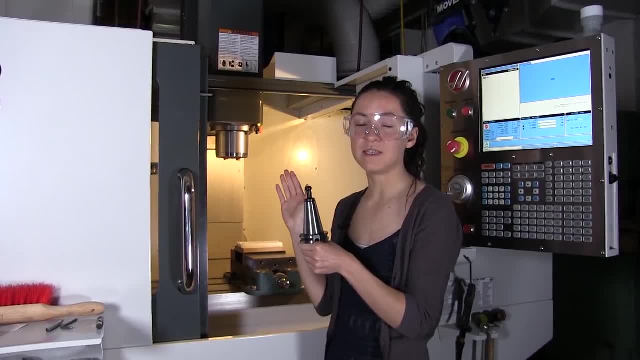 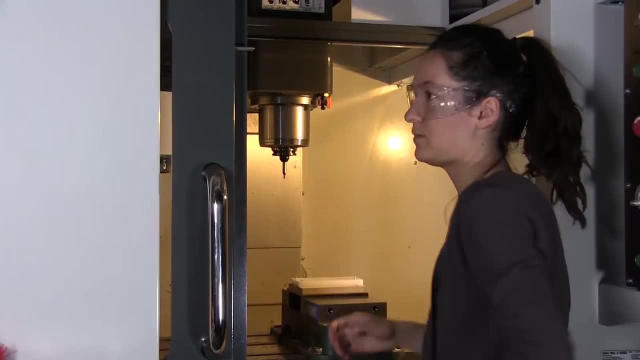 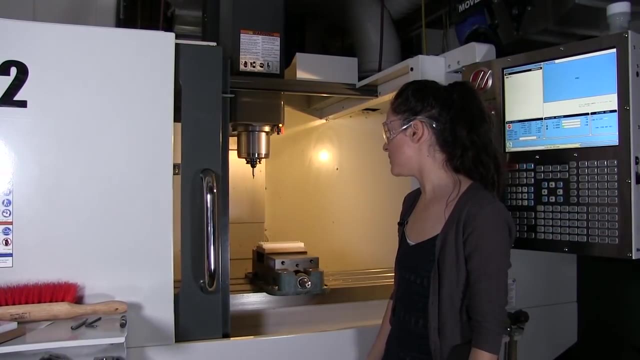 So line up the notches, press the button. When you release it, it will pull it into the spindle, Just like that. Now that the tool is in the spindle, we're going to need to move it into the location to start finding that back edge of the part. 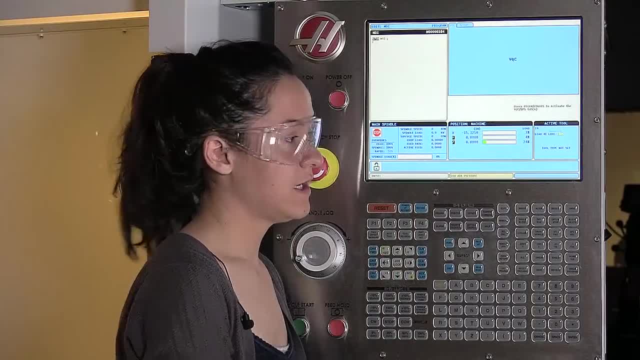 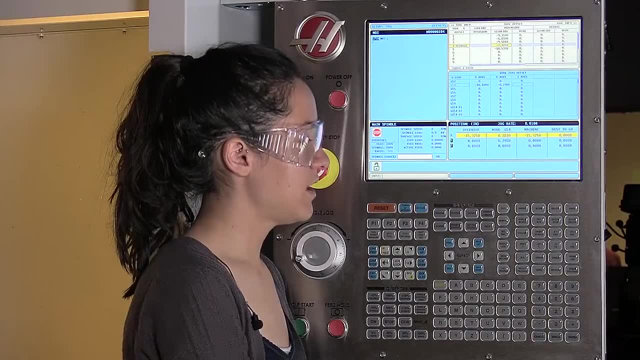 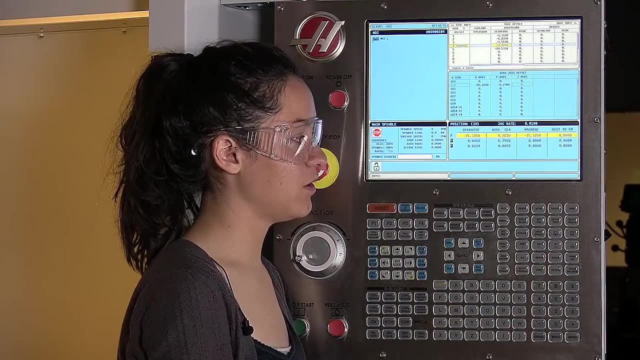 To do that, I have to get into a different mode. I'm going to go right to this handle jog mode that will let me move the table and spindle around. Next to that handle jog is the increments at which you're moving it. We just start at this: 0.01.. 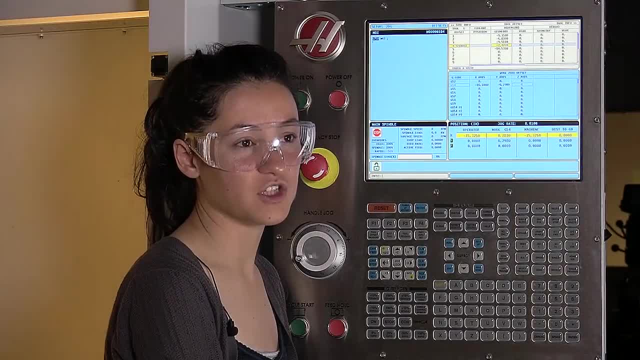 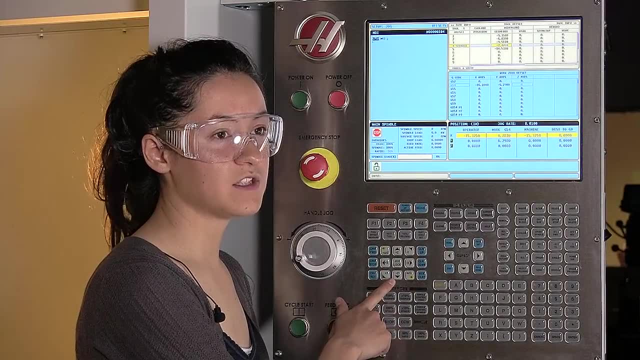 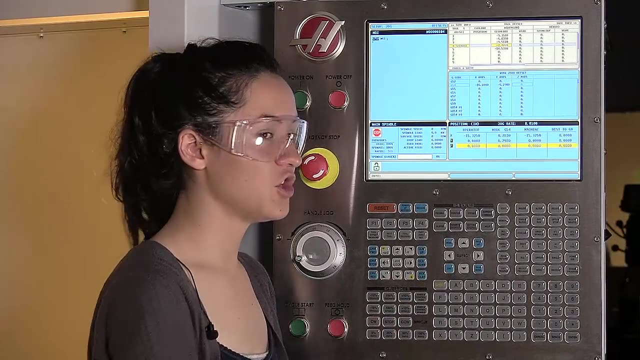 That's about as fast as we move, so we don't risk crashing the spindle into anything. Now over here you have your X, Y and Z. Plus or minus, doesn't matter, But you'll determine the direction with this dial. So X moves the table left and right. 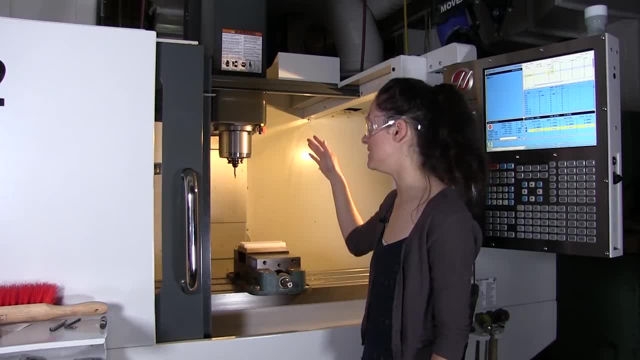 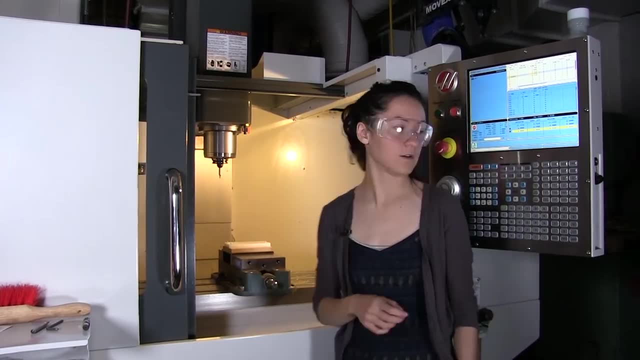 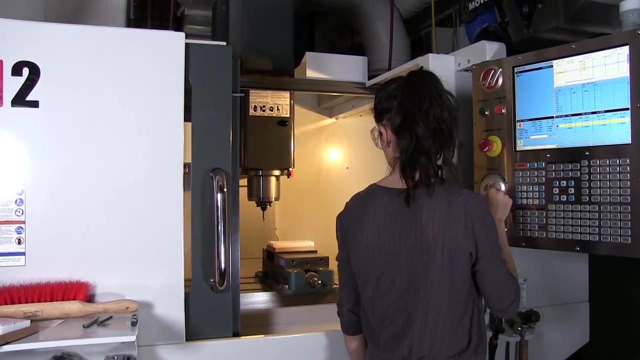 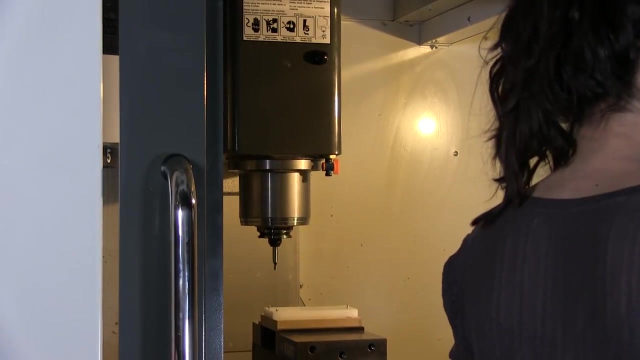 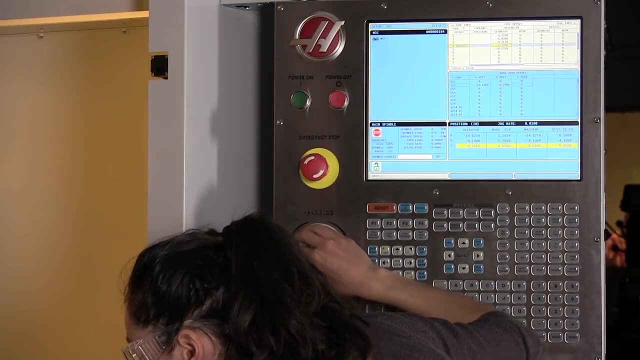 Y moves the table forward and backwards And Z moves the spindle up and down, So I'm just going to move it until the edge finder is right behind this stock here. You've got some diyorumels here, And when you get to zero, 1, 1,, 2, 2, 3, 4.. 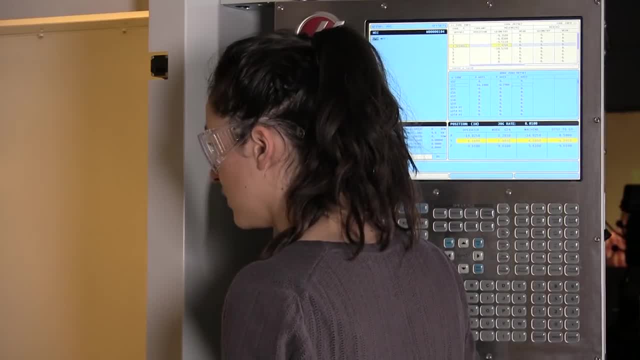 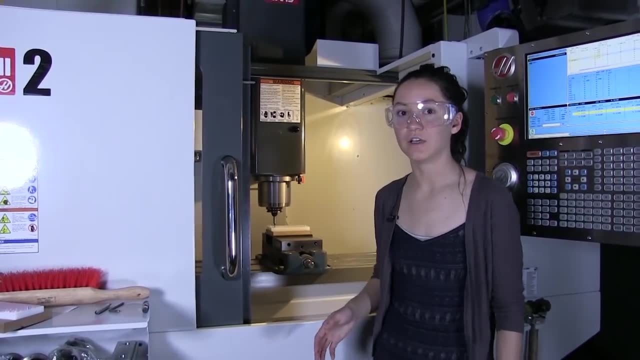 We move the table 1, 1,, 2,, 3,, 4,, 5,, 6,, 7,, 8,, 9,, 10,, 11,, 11, 12.. Now that the spindle's in a good location to start, I'm going to start the spindle up moving. 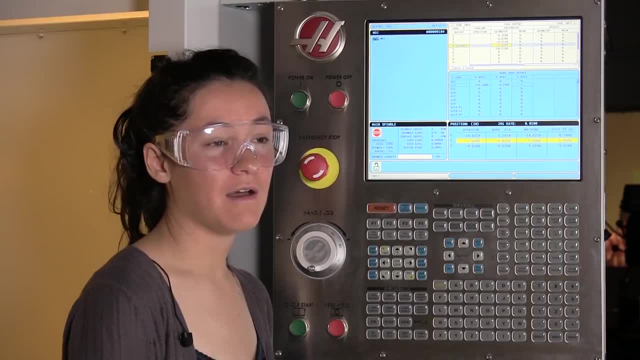 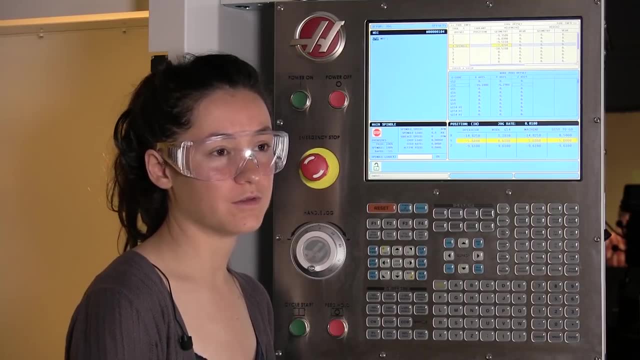 An edge finder works best at 1,000 RPM. However, the door of the machine has to be closed if you're running at over 750 RPM, Because it's easier to see what's going on with the door open. we're just going to run. 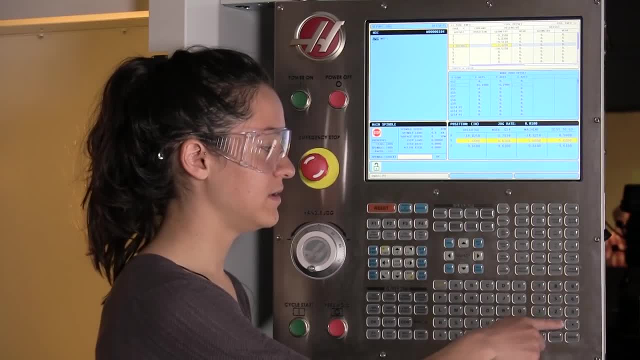 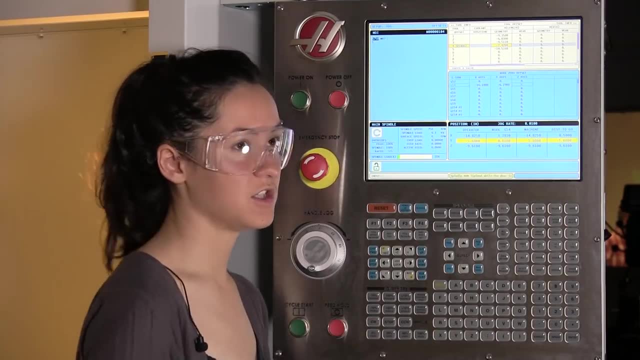 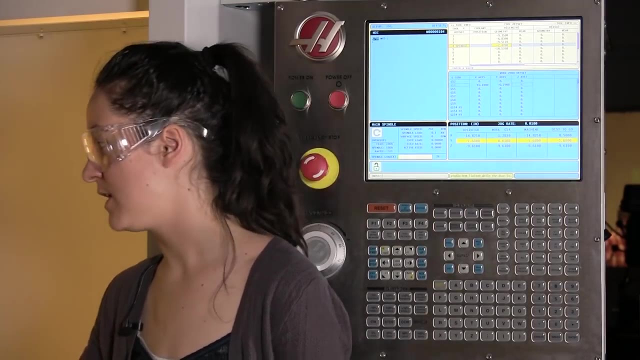 it at 750.. To do that, I type in 750 to this keypad and then I press clockwise CW to start up the spindle. Since this is already wobbling, you don't have to flick it. but if it was concentric? 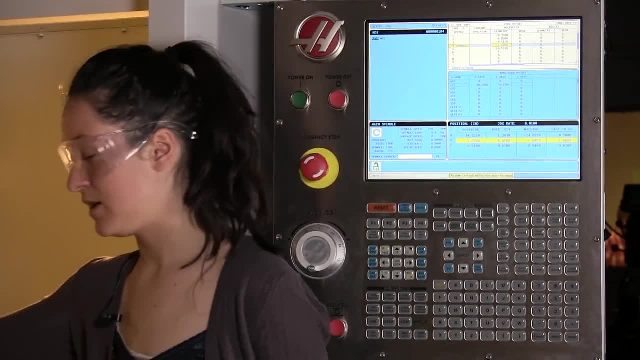 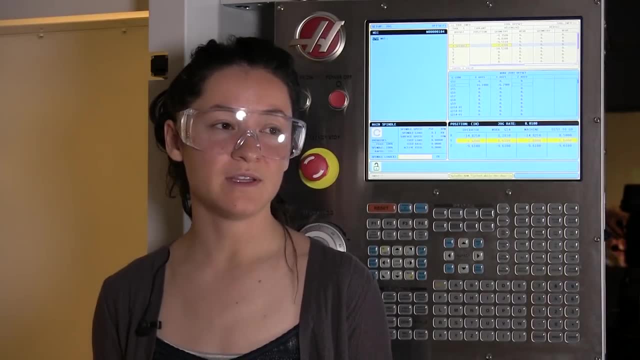 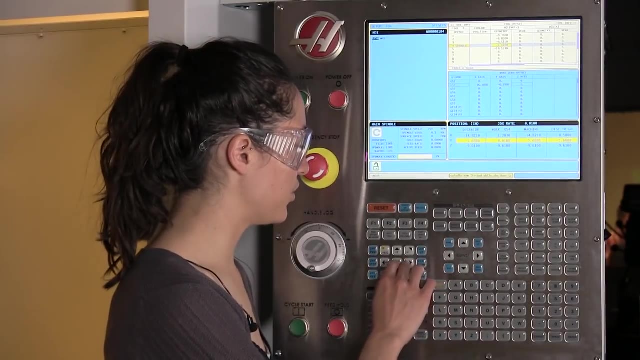 to start with, like that. you just have to reach in and flick it so it starts wobbling. Keep in mind, this is the only tool you're going to touch when it's spinning. Now that it's all started, I'm going to bring it in in the Y direction. 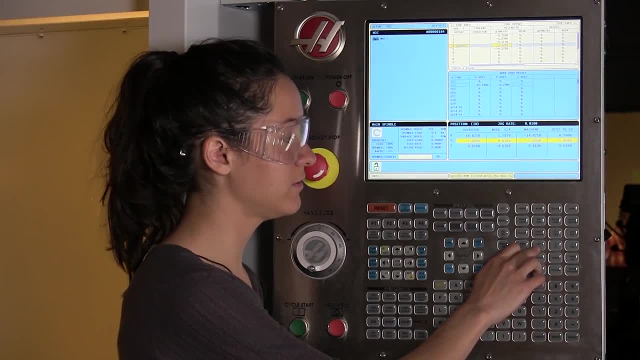 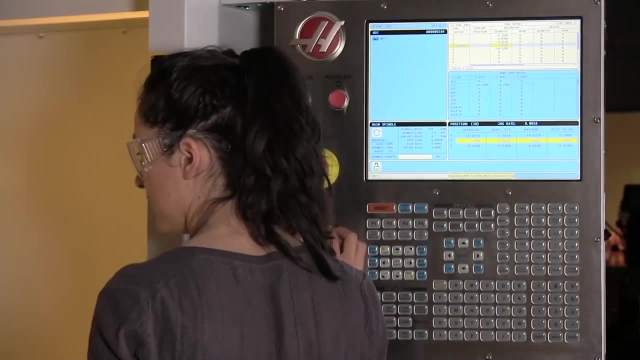 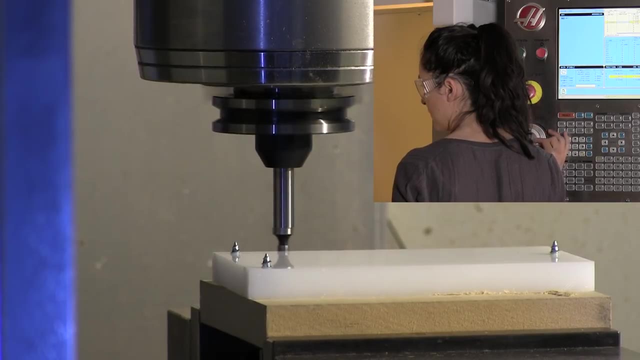 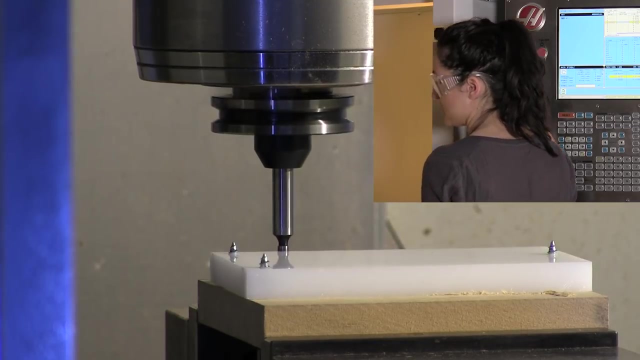 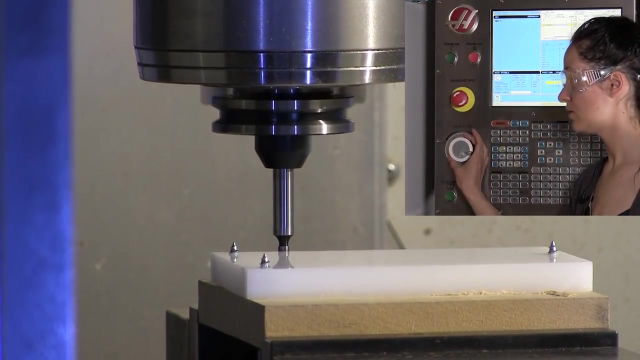 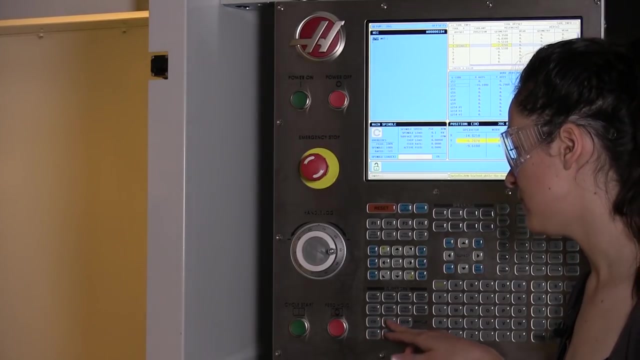 Since I'm close, I'm going to go down one increment lower, just so I have more precision. Okay, It's starting to go concentric now. Now I'm going to go slower Until it just steps off like that. I'm going to stop the spindle here with this stop button right next to clockwise that. 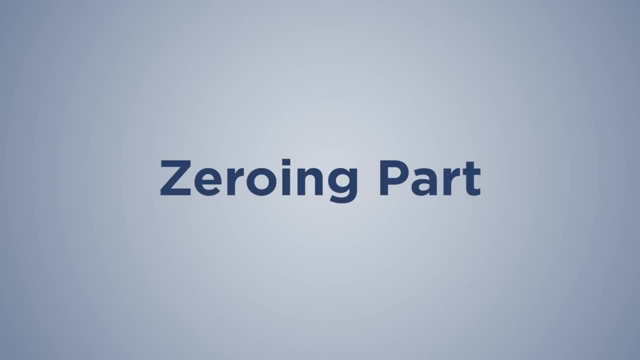 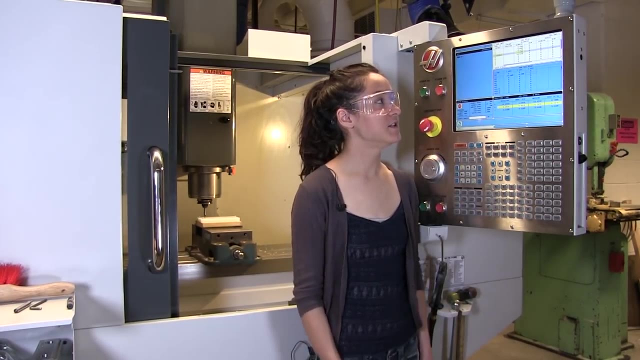 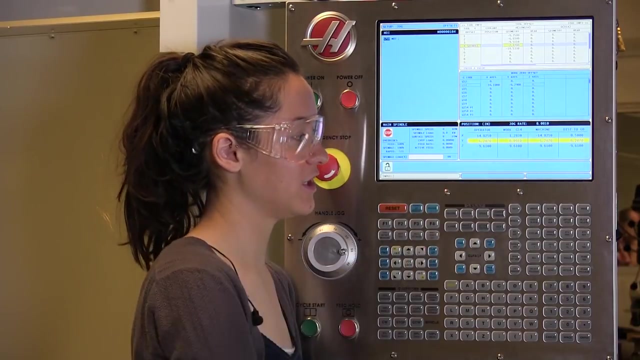 started it up. Now that you've found the edge of that part, you're going to want to tell the machine where that zero is. To do that, we're going to want to switch into this work zero offset menu and work in this G54 line here. 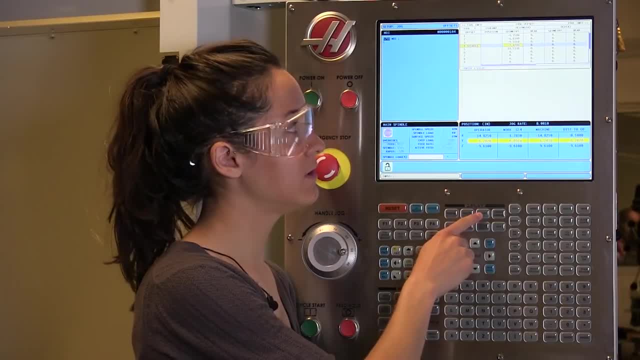 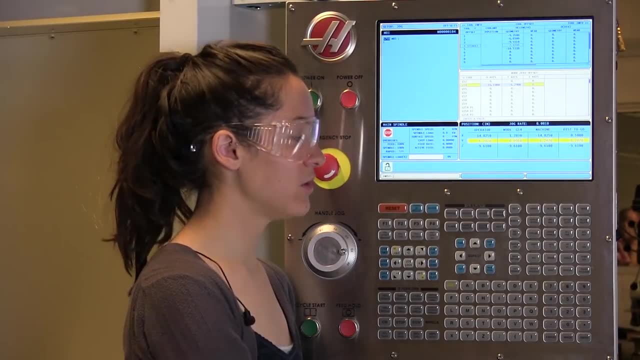 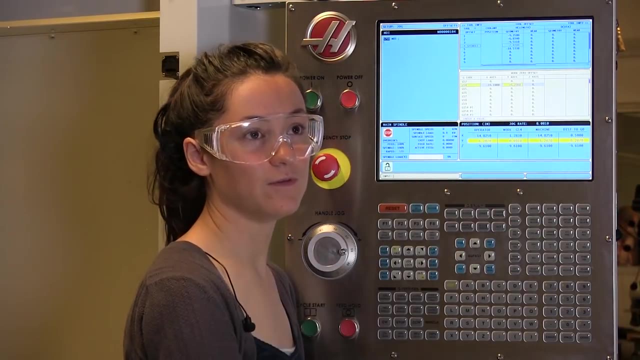 To switch to that menu. you're going to press this offset button. That will highlight this menu we're working in. We just zeroed it in the Y direction, so I'm going to use these cursor arrows to make sure that yellow box is in the Y axis and in the G54 line. 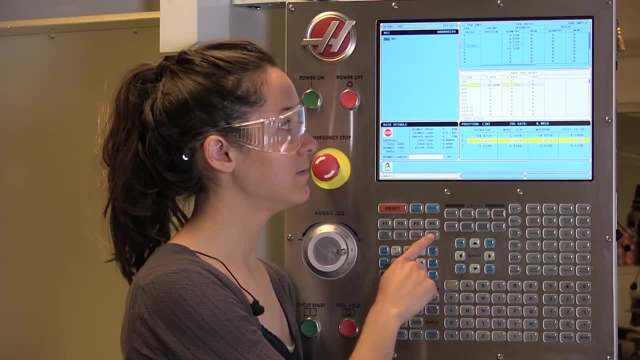 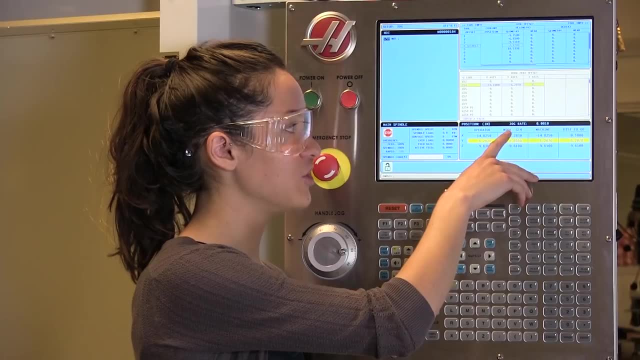 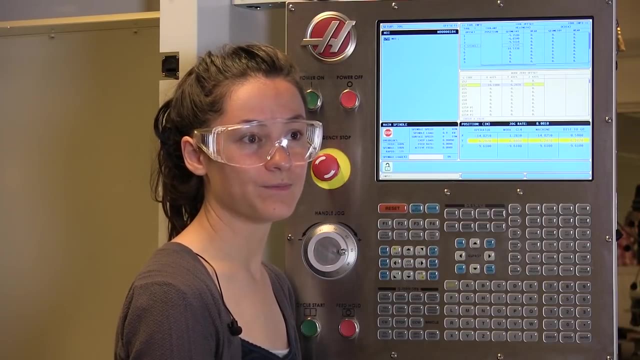 Now I'm going to use this part zero set button and that will zero it out where that tool currently is. You can double check in this work: G54 and Y. That's all zeros now, because we just zeroed it there. Now we have to compensate for the radius of the tool. 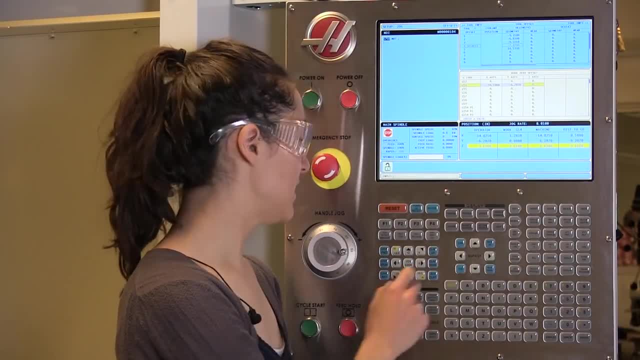 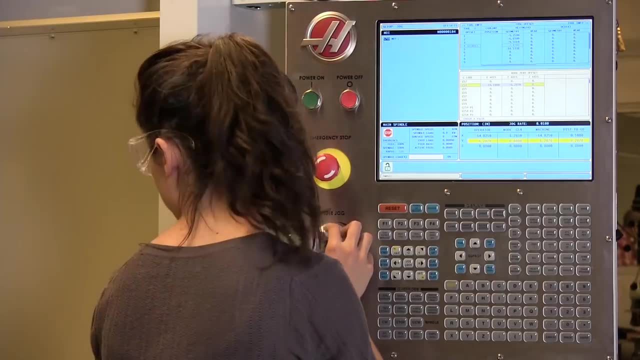 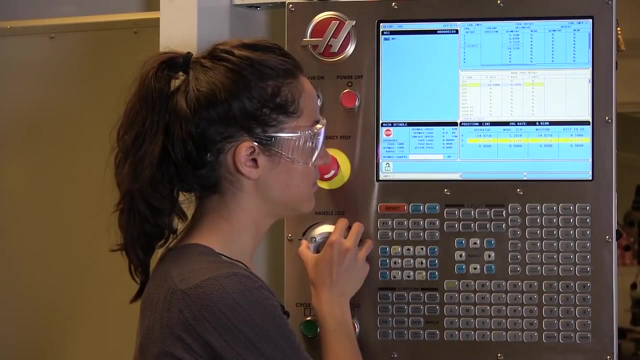 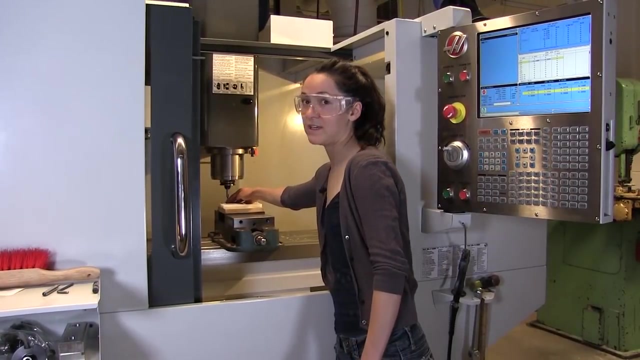 An easy way I like to do this is to just bring the spindle up away from the part and then bring it over in the Y direction until that is point one. Double check That the tool center is over the edge of the part and not further away. 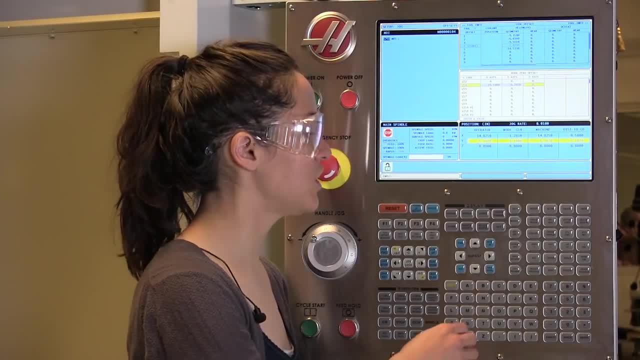 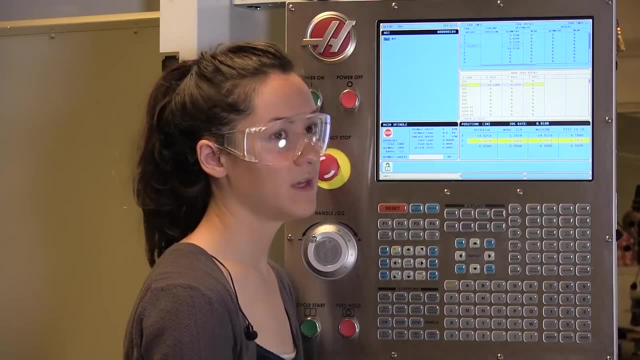 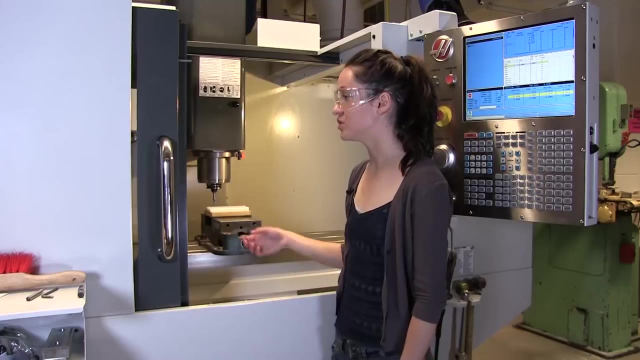 Now that I have this new zero where the center of the tool is over the edge, I'm going to go back into that Y axis and re-zero that with this new position. That's how you compensate for the radius of the tool. The same process will be used for the X direction. 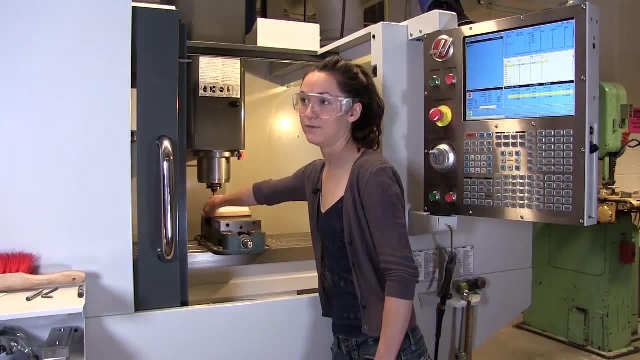 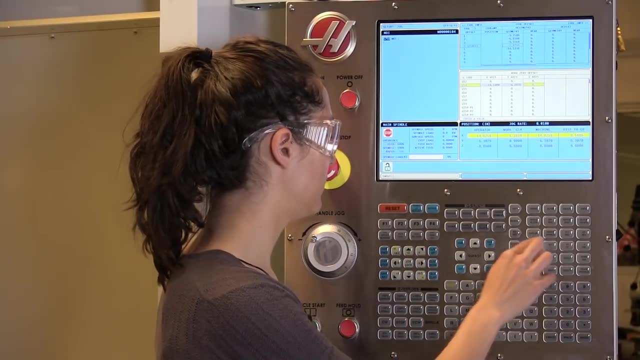 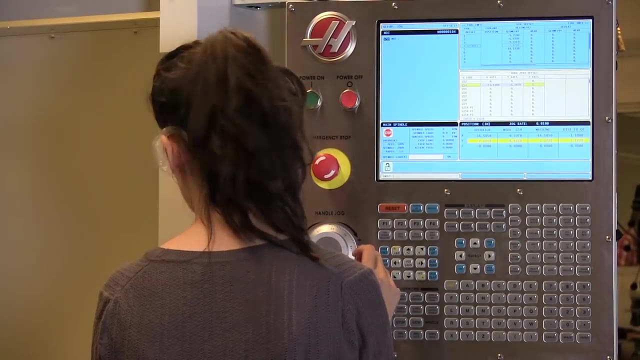 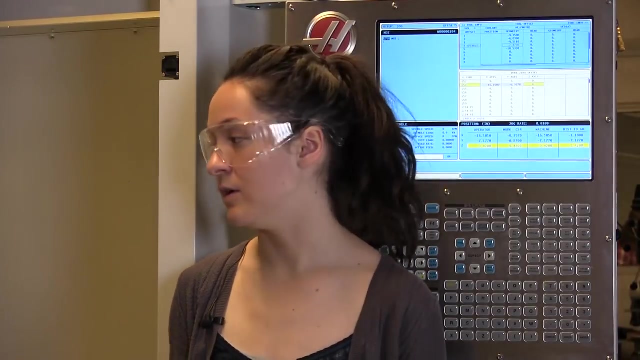 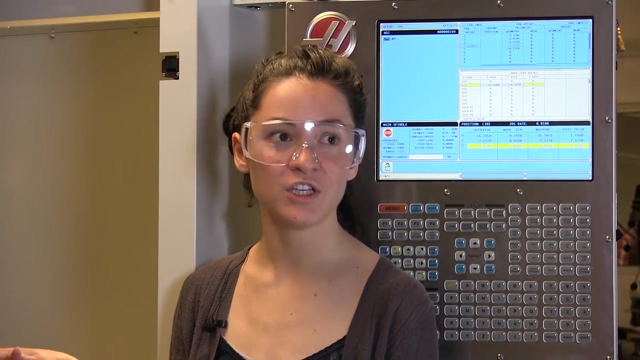 We're just going to bring the edge finder over to this side and find off of this edge here. The only difference with finding the zero on this edge is that when the tool goes concentric and breaks off, it's going to break off towards the back of the machine instead of towards. 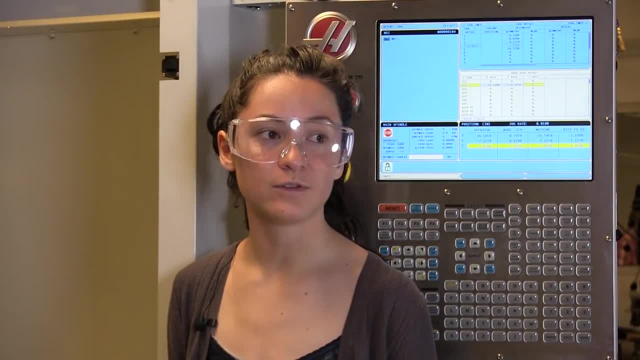 the right, like we did on this back edge. That's going to make it difficult for the tool to get out of the way and then break off over to the back to see if you're looking at it straight on. so what i like to do is when the tool goes concentric. 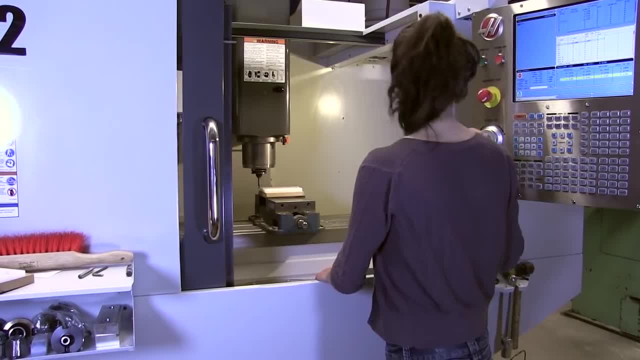 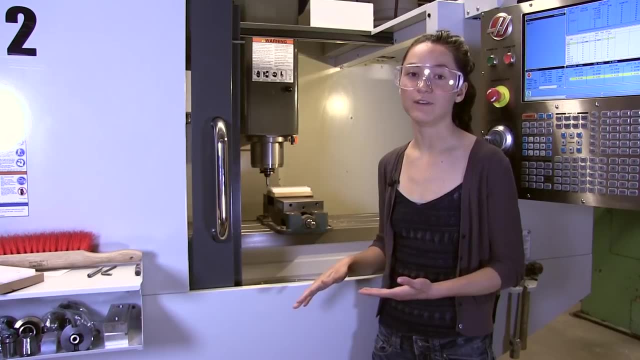 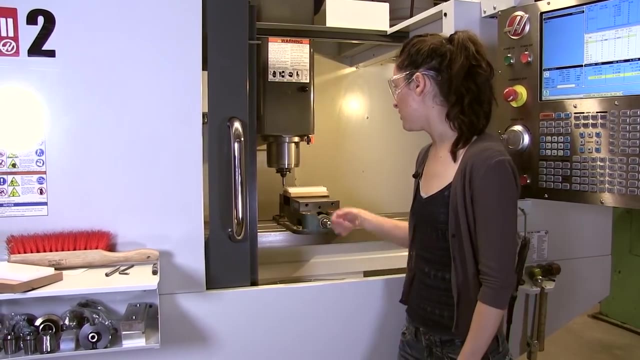 i stick my head in the machine and, with one hand, keep moving the dial, but be looking at it from the edge so you can see it break off easily. now that we're in position, i'm just going to start the spindle up again, make sure it's wobbling and then start bringing it in. 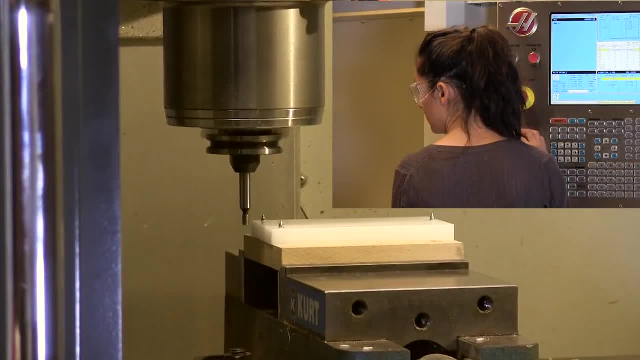 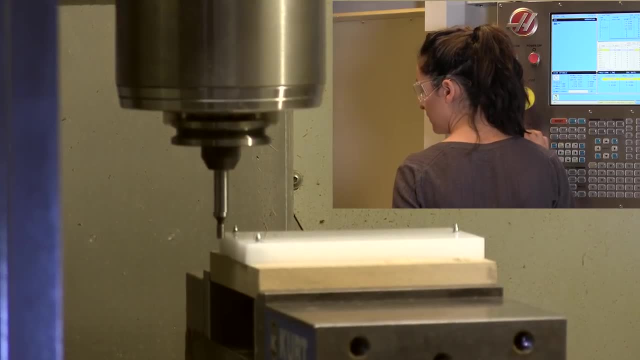 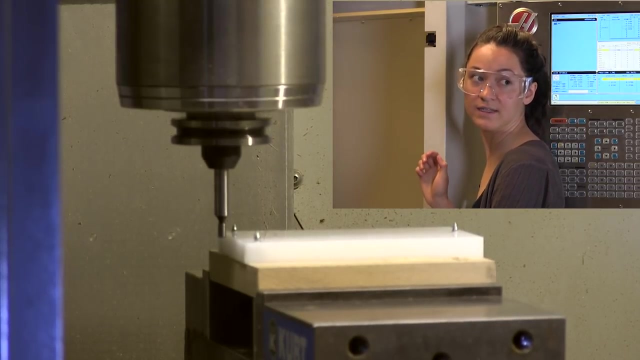 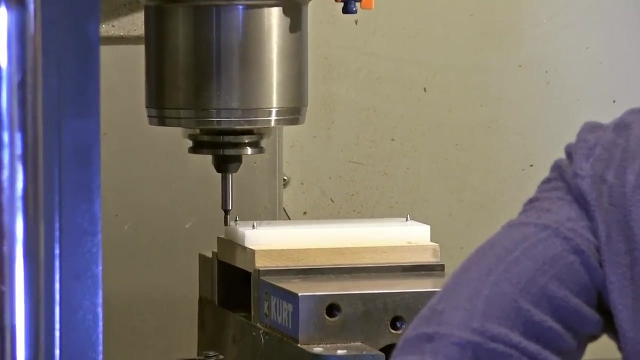 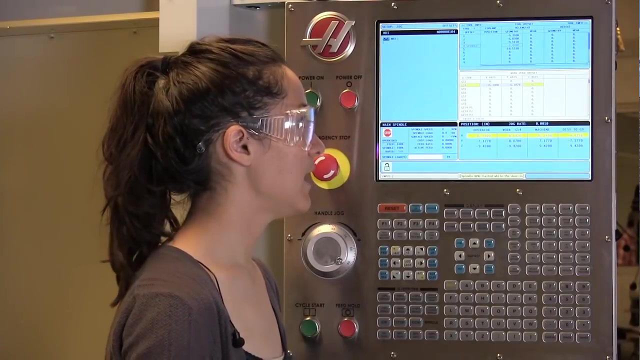 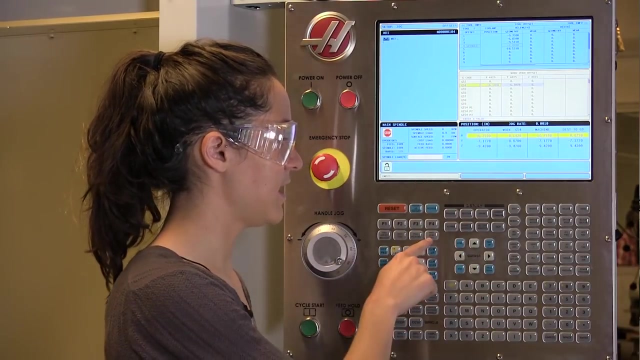 with a smaller increment. now that it goes concentric, i'm going to look in and make sure it breaks off. right there it broke off. so now i'm going to stop the spindle and then zero this new position in the x. so i'm going to make sure i'm highlighting that x-axis and then part zero set. 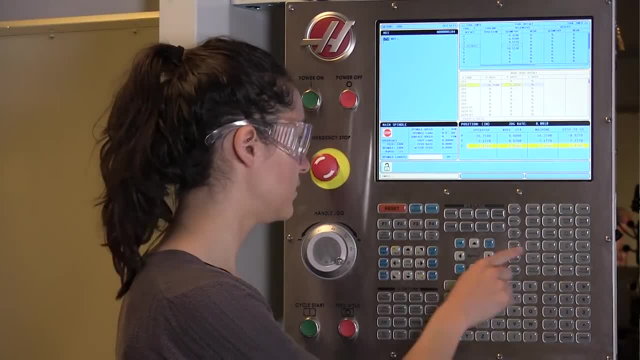 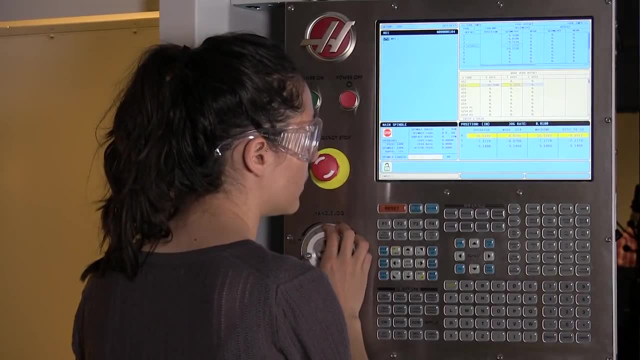 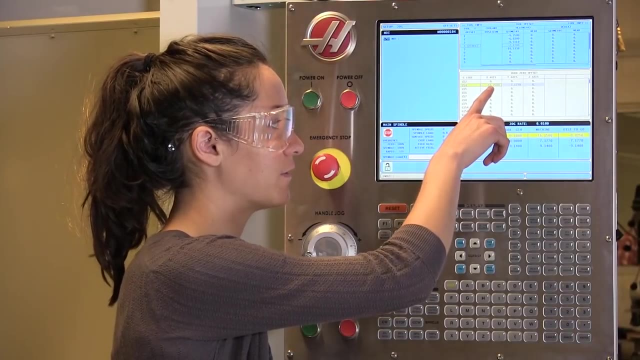 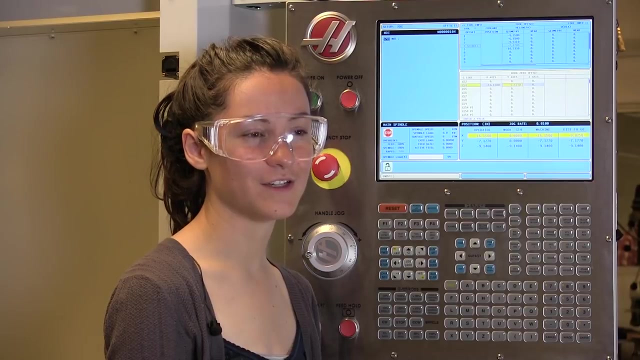 now just to compensate for the radius of the tool, make that 0.1. now that you've compensated for this radius, i'm just gonna zero over that x. in this new position, now that you have both your x and y zeros set, you have to set the z zeros for every. 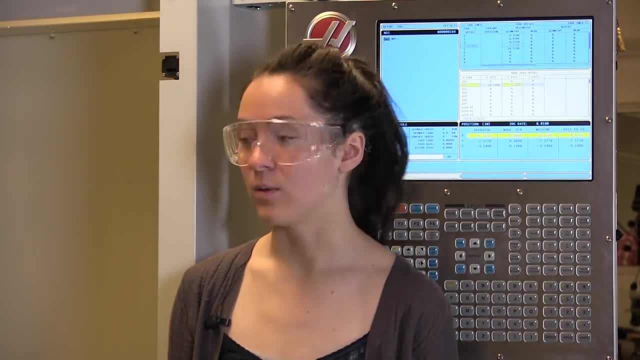 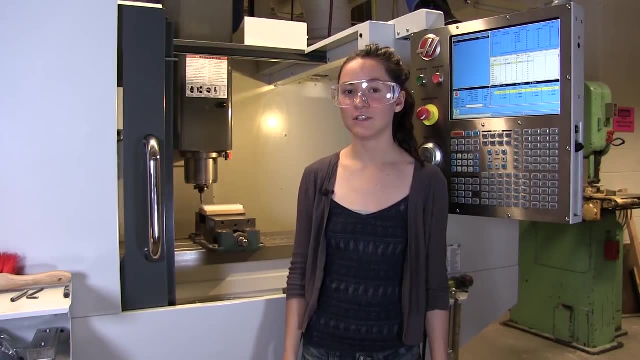 tool you're using in the program. this just tells the machine where that tool is just going to start cutting into the top of your stock. so, to zero in the z direction, you're going to have to change tools to one of the first tools you're using. 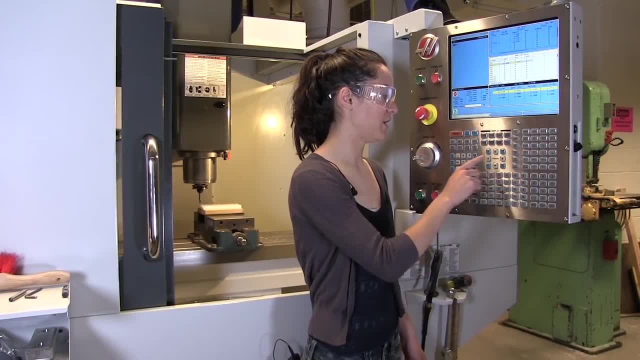 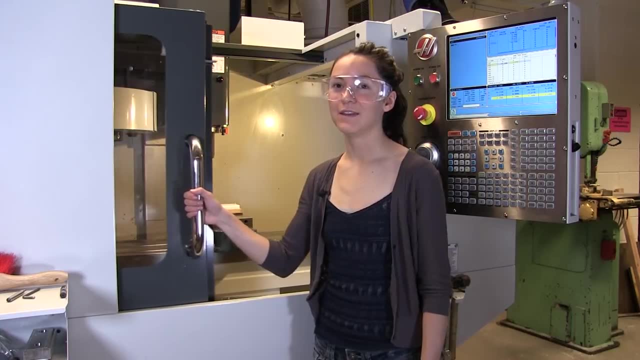 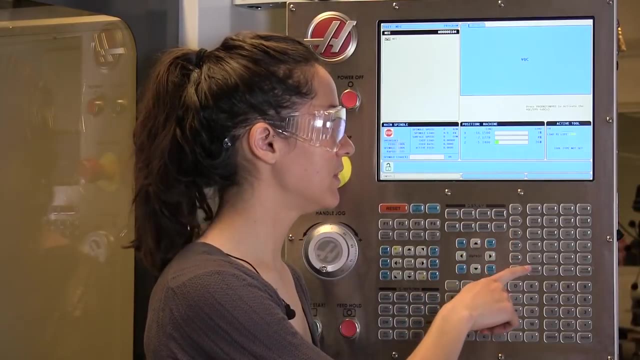 so before i let it do an automatic tool change, i always bring the spindle away from the part to make sure that it has clearance. then i'm going to shut this door so it can do the tool change. now get into the correct mode and then we're going to want to go to tool one. 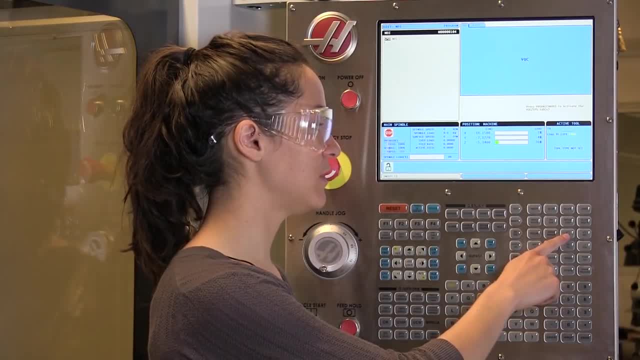 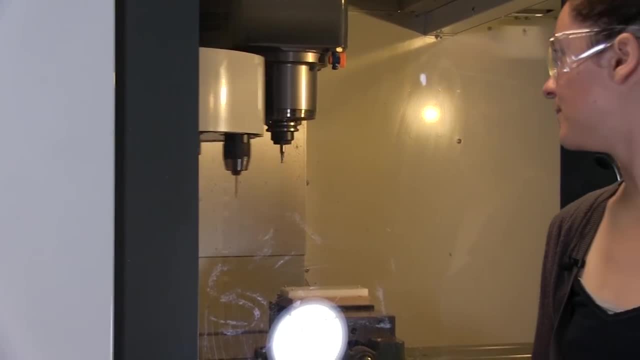 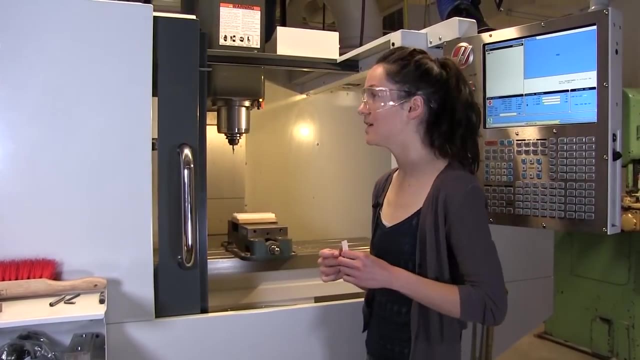 so t for tool one, for the first tool, and then we're going to want to go to tool two, and then we're going to want to go to tool three, and then we're going to want to go to tool three to zero a tool we use, this paper test. we're just going to put this down on top of the stock. 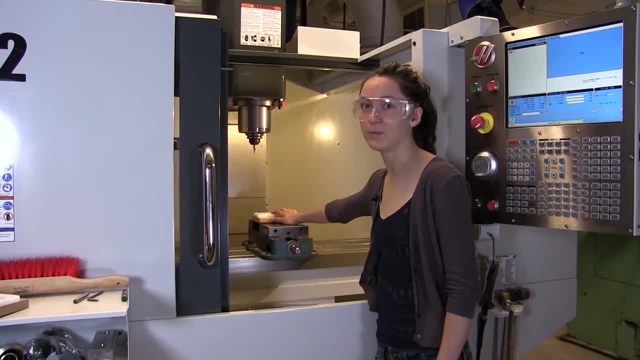 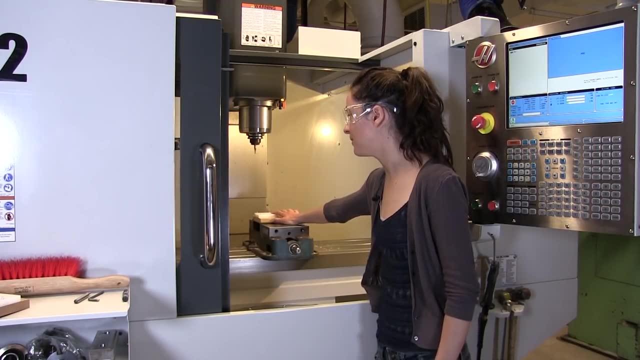 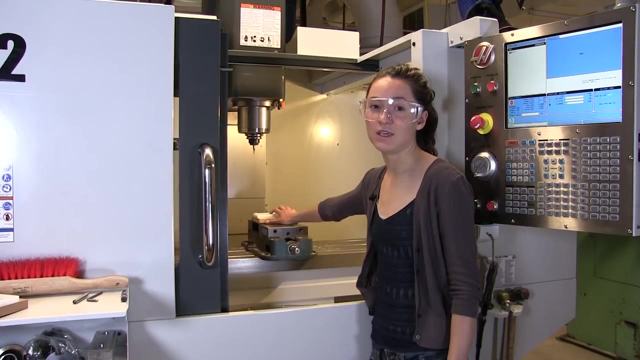 bring the tool over and down until it's right above this paper and then slowly move the spindle down- it's not going to be moving at this point- and move this paper around until you feel the spin, the end mill dragging on that paper in the stock, not so much that you can't move it, but just a little less. so you feel quite a bit of friction. 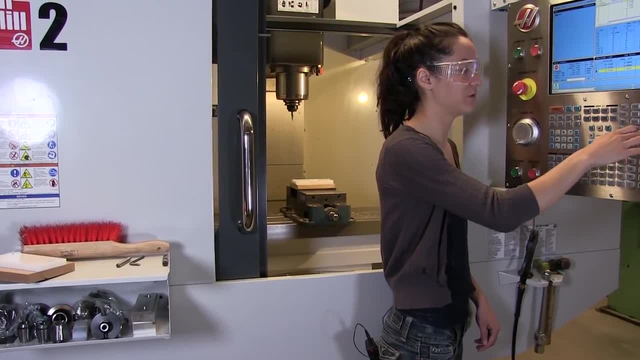 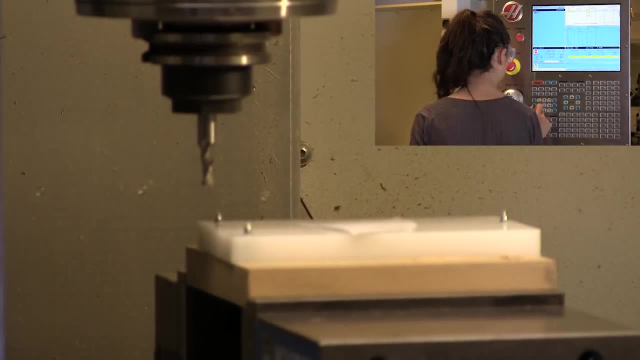 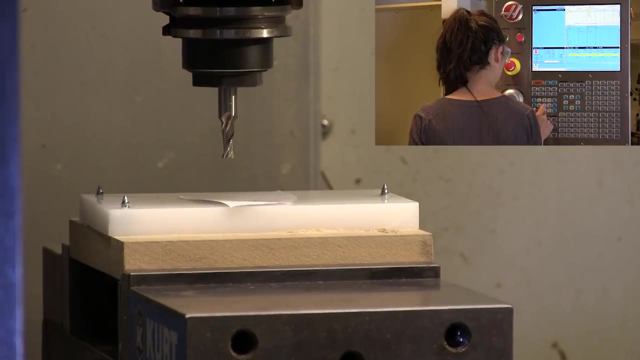 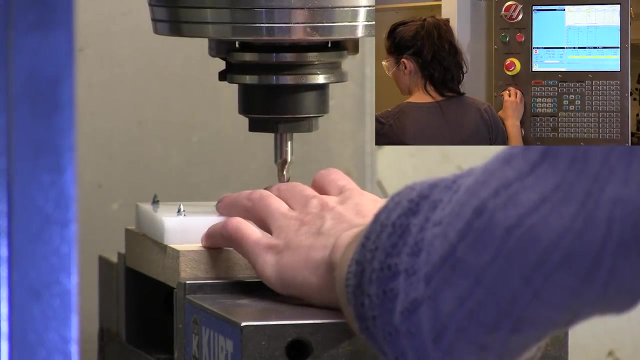 make sure you get in the correct mode to move the table and spindle around, and then we're going to want to have our tool at a reasonable angle, and then we're going to want to have our tool out of the way. then we're going to have our tool in the right position. 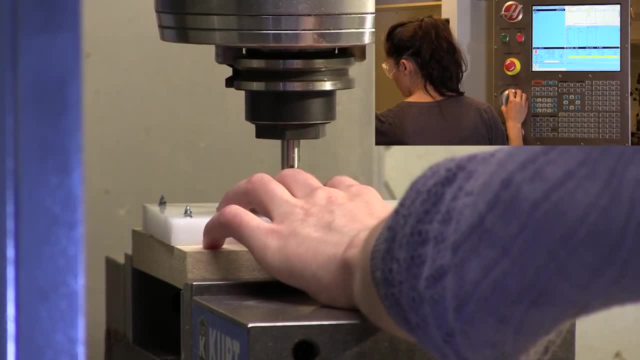 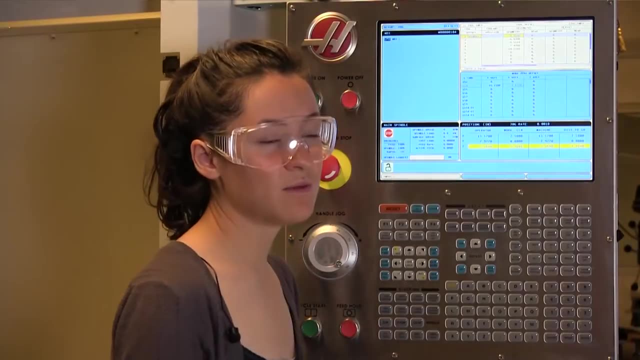 so that it can move in a lot of directions, and then you want to get the hold most of the time. once you're in there, you can sling it from this side, you can place it in a lot of different angles and again it's the wrong position. 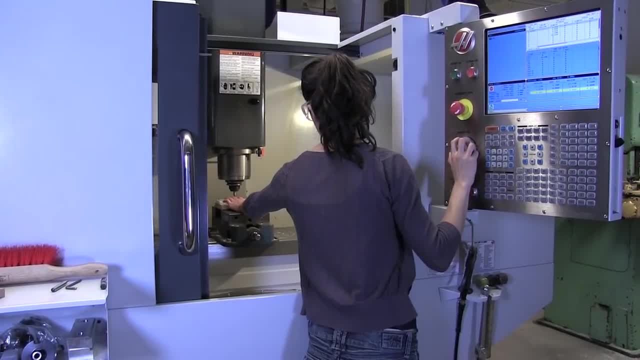 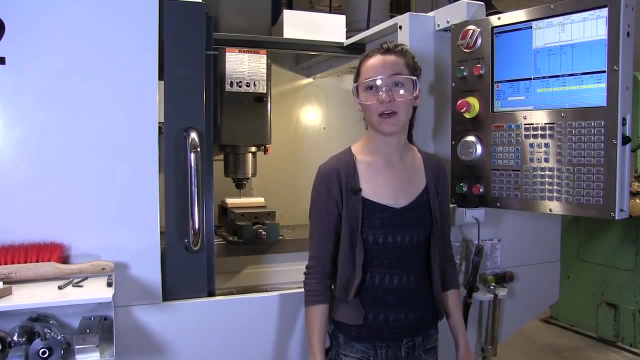 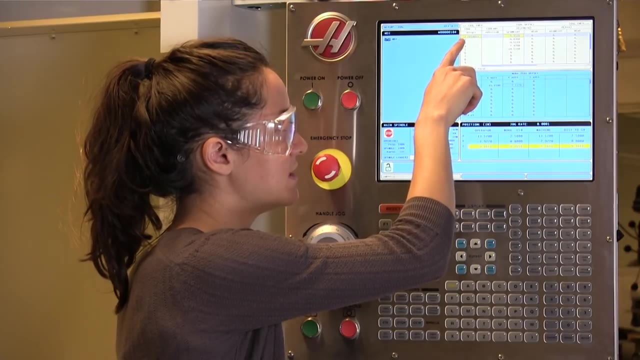 sometimes with the paper test, it's necessary to use the very smallest increment. you can use the little finger rinse for the most part. Now that I've found the top of that stock, I'm going to tell the machine where that location is. Up here in this tool, offset menu spindle is next to number one, which is the tool that we're currently using. 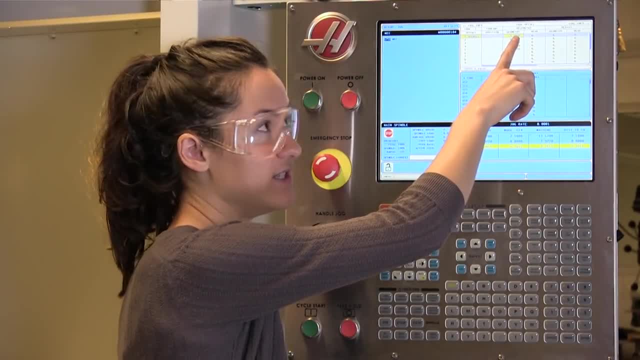 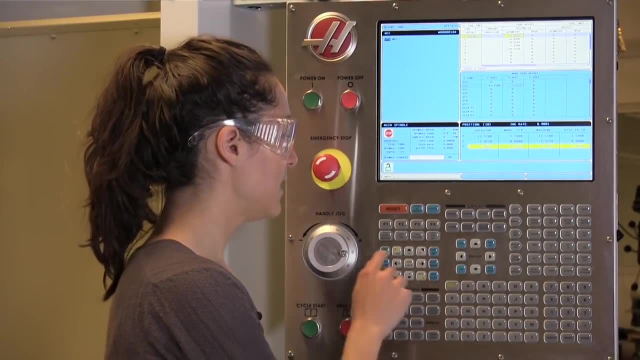 And then in this geometry column is where you're setting your Z zero. If this isn't highlighted with the yellow box, just use the cursor arrows to get over to that box, Then press tool- offset measure and that will zero that in this new location. 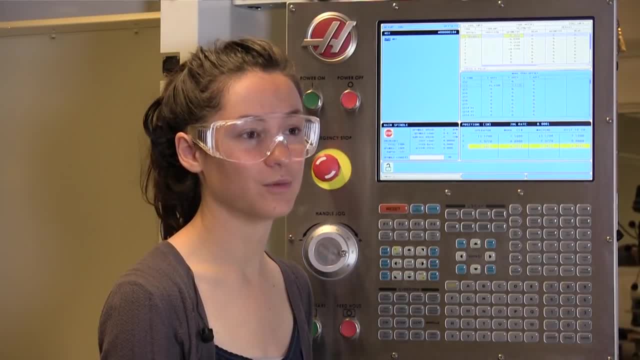 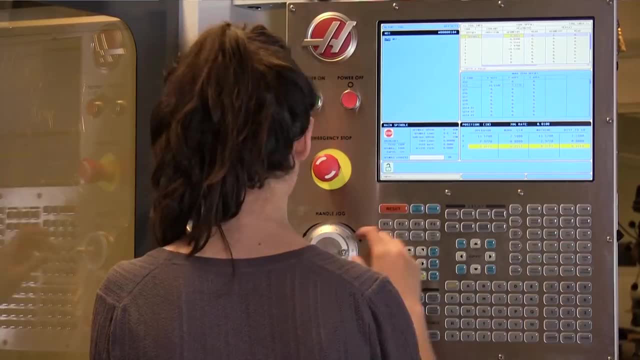 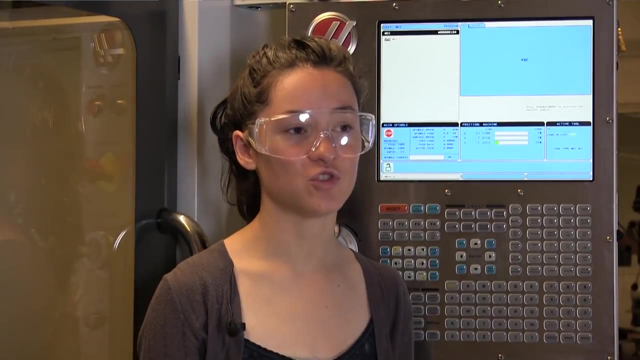 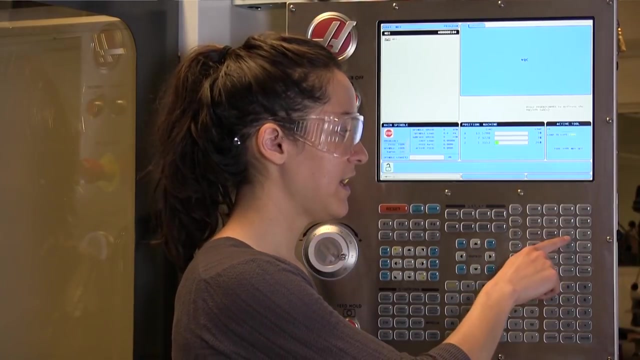 This process needs to be repeated for every tool you're using in your program. A shortcut to switching just one tool ahead is to be in this correct mode and then, instead of typing the next tool, ATC forward will take you one tool in the next direction. 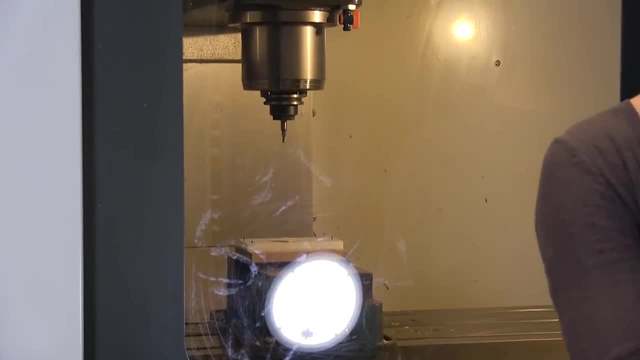 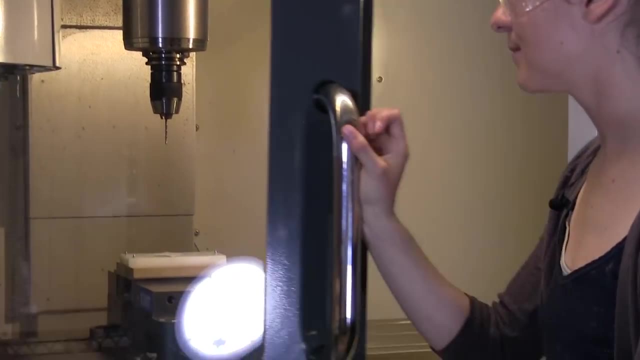 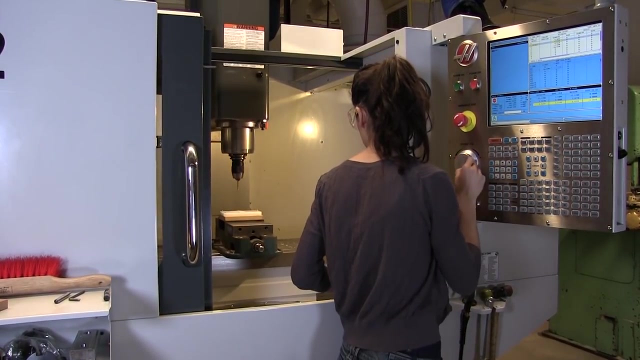 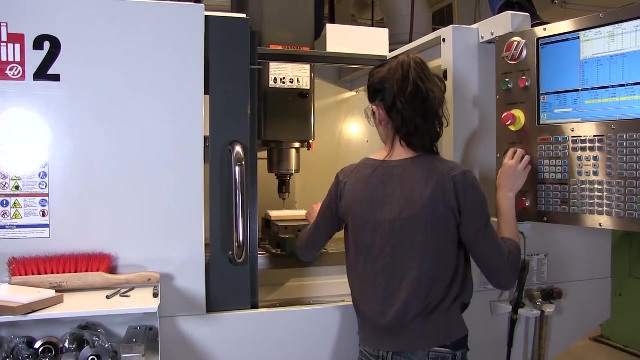 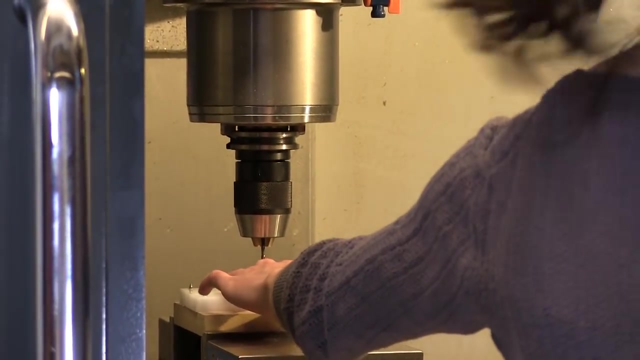 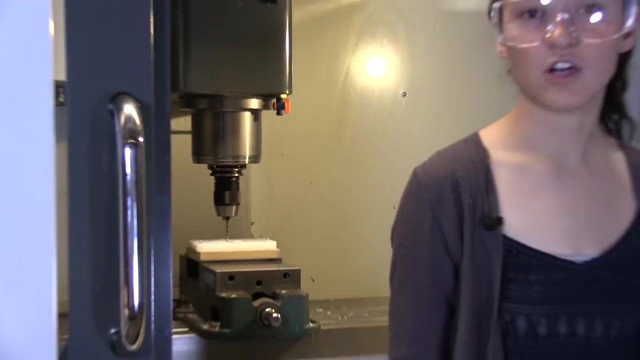 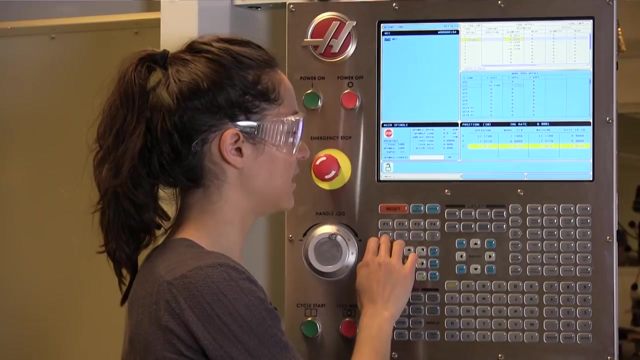 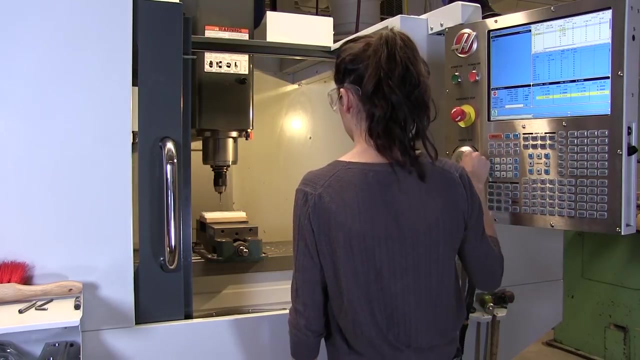 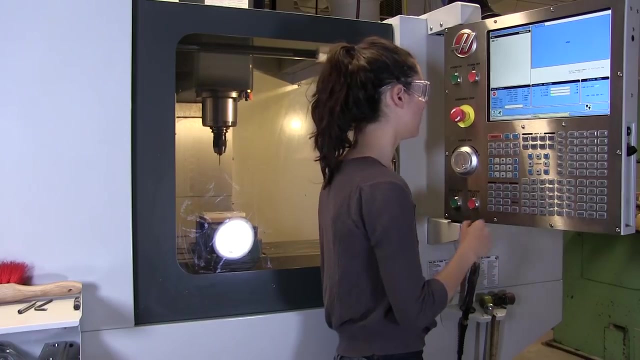 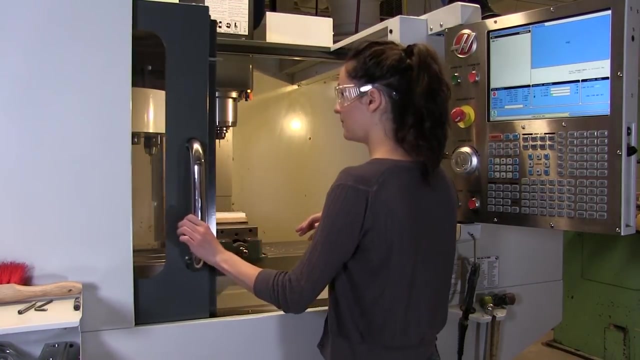 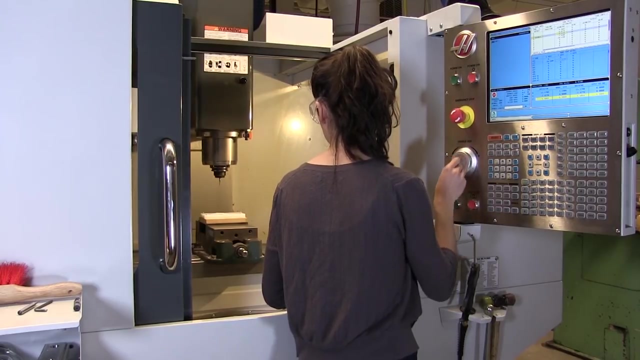 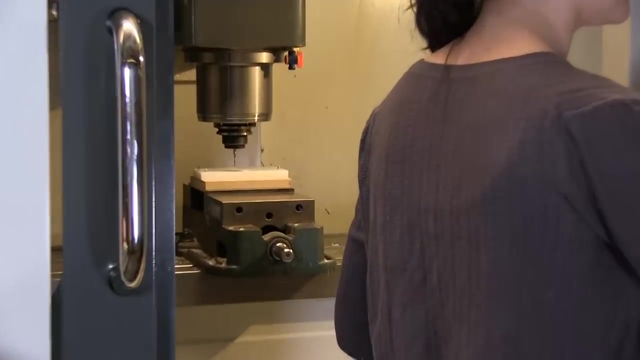 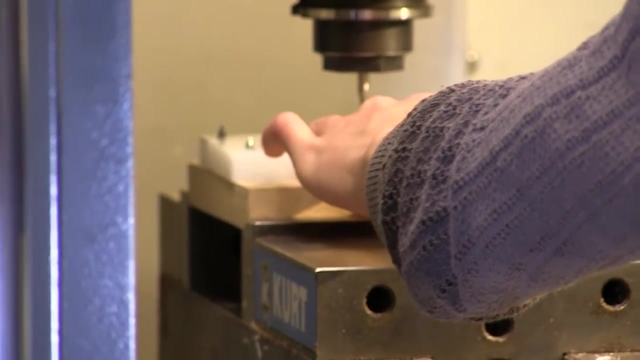 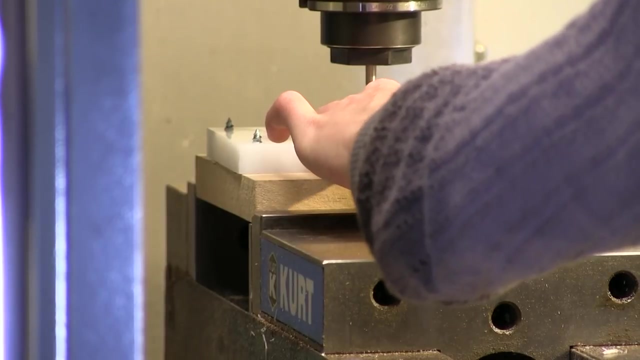 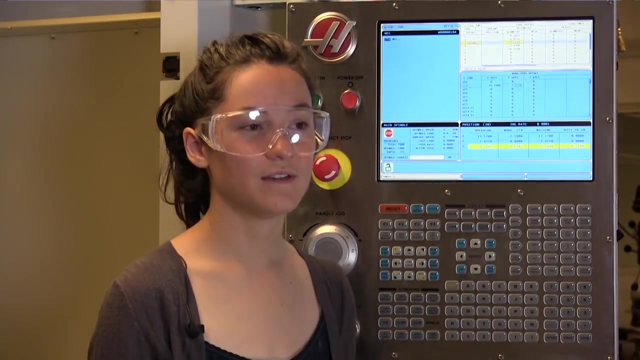 and ATC reverse will take you one tool back. I found that top of the stock Now spindle is next to two because we're in the second two. Go ahead and zero that out. Now that I have zeroed all the tools that we're using, you're essentially ready to start. 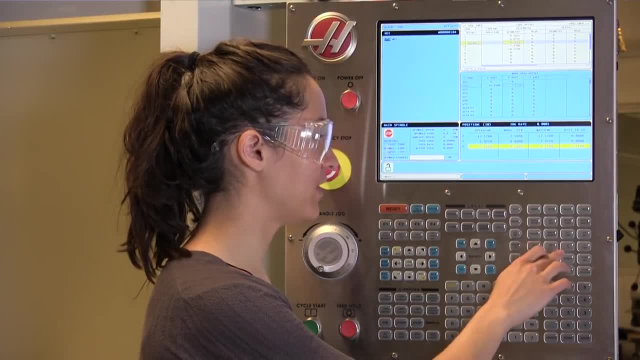 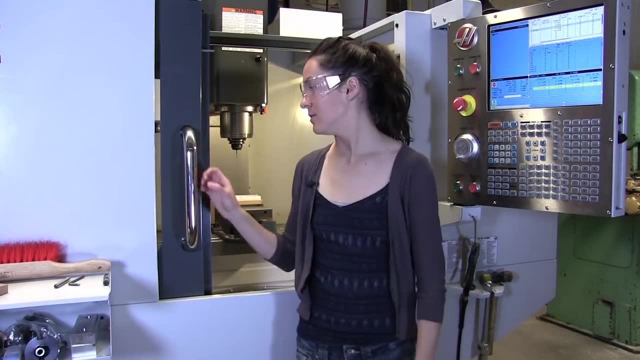 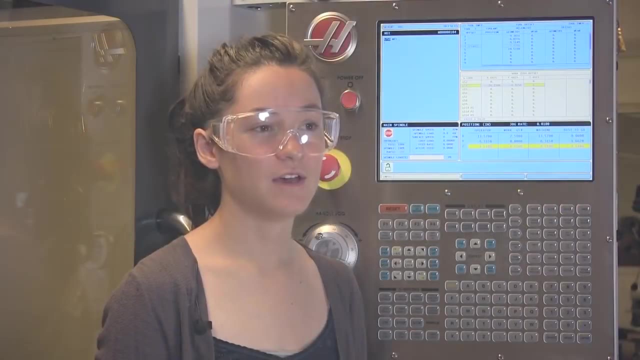 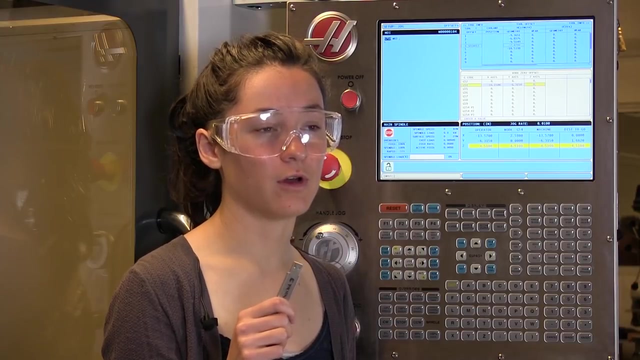 running your program. So before it runs, I always bring it away from the stock. Now that everything is zeroed, you're going to want to put the program into the machine. Your G-code from your Mastercam file should be saved on a USB drive. 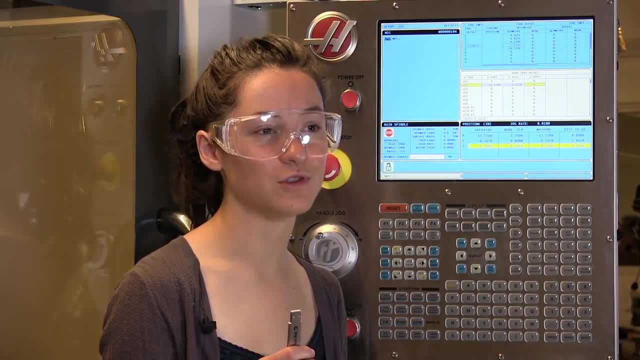 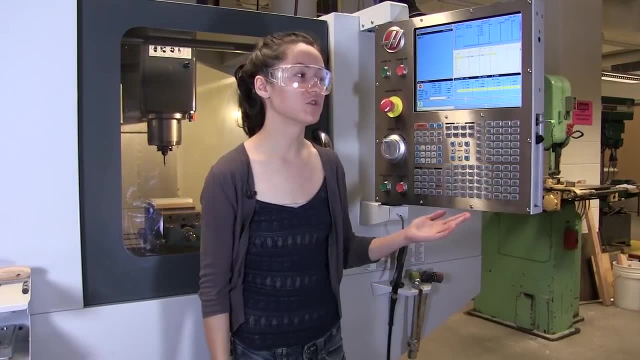 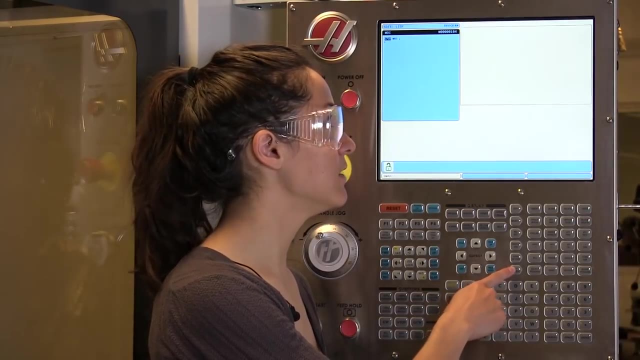 To learn how to make this G-code reference the Mastercam, Insert the thumb drive in the edge of the machine and then to bring it up. I'm going to use this list program button here. That will get me into the correct mode. 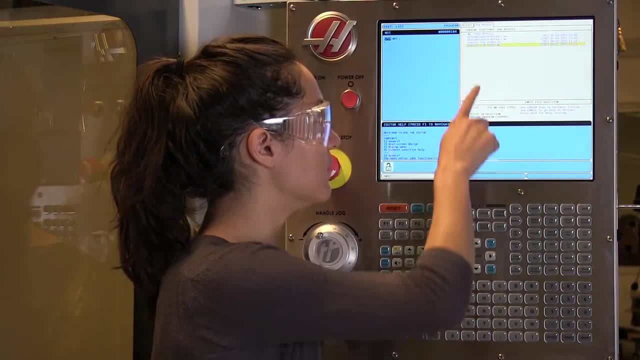 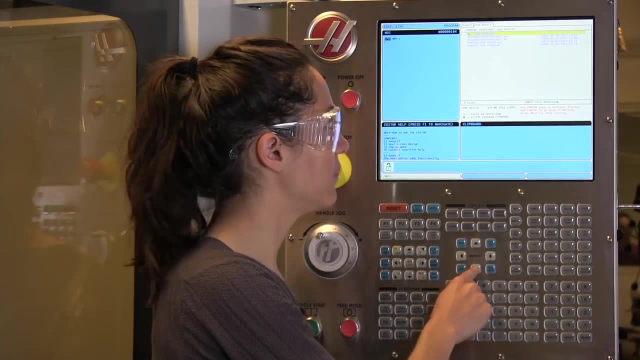 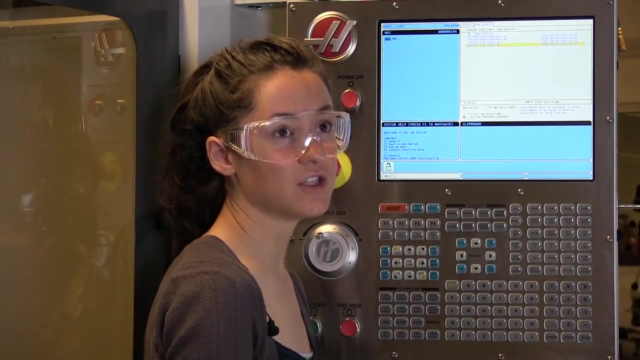 Currently I'm in the USB device. If I wasn't and I was over in memory, you would just use your cursor arrows to come up to the top tab to move back and forth. I'm going to select my file. It should have the nc extension, not the err. 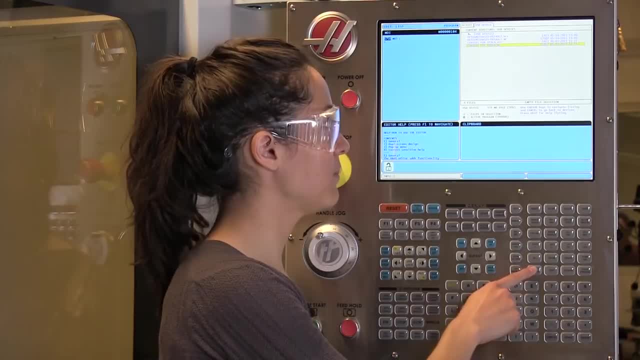 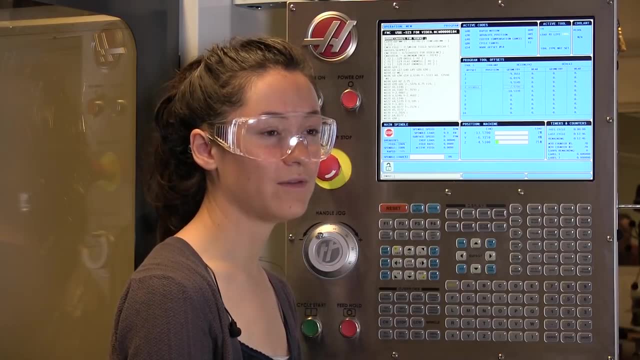 To bring this file up, I'm going to press select program and that will grab that file. Before you run your file, you're going to want to do a settings graph of it to make sure everything looks correct. To do that, you're going to press the settings graphic button twice. 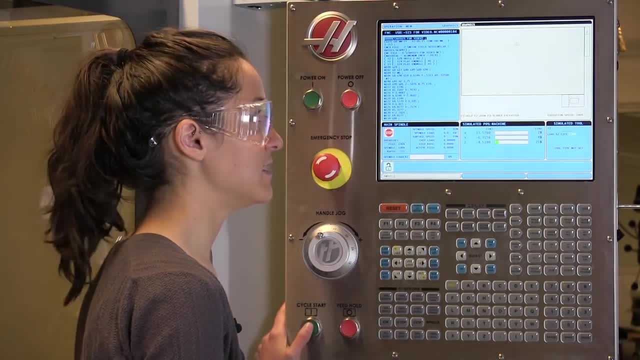 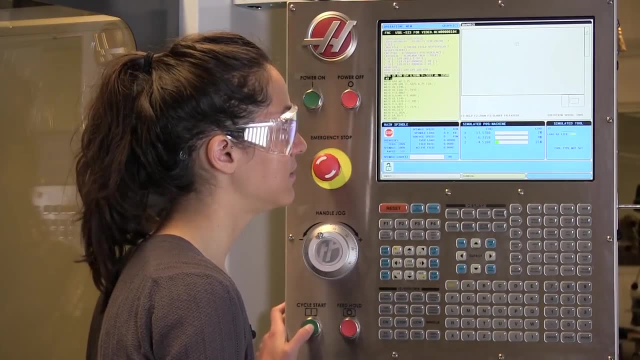 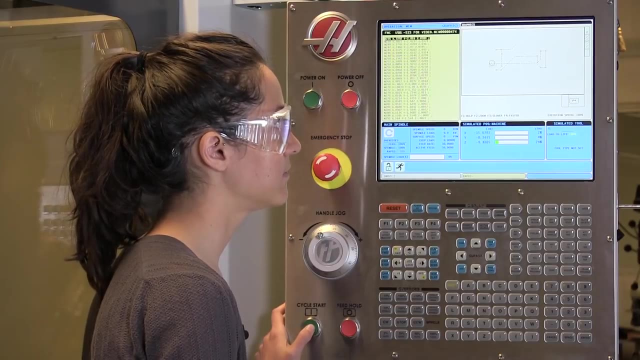 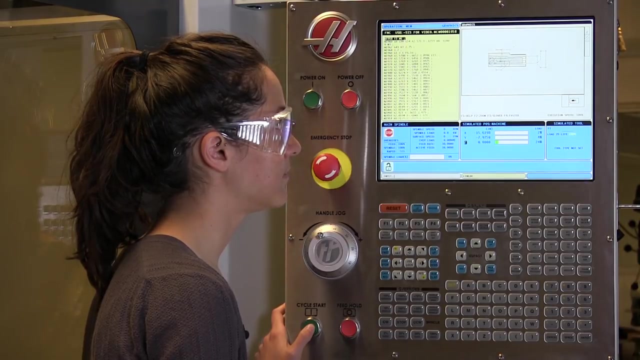 Then the cycle: start. green button to step through the file. It's going to show up on this screen here all of your toolpaths: The X's mark where holes are being drilled, Dashed lines are rapid motion and solid lines are cutting paths. 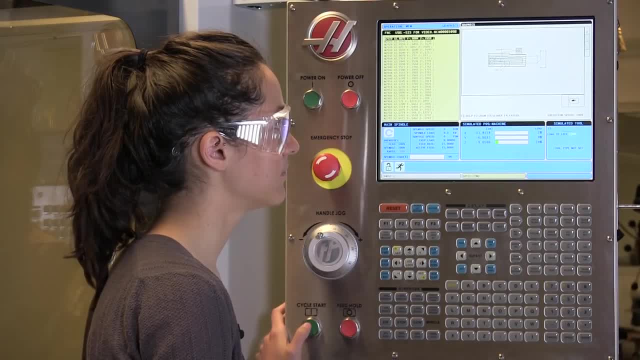 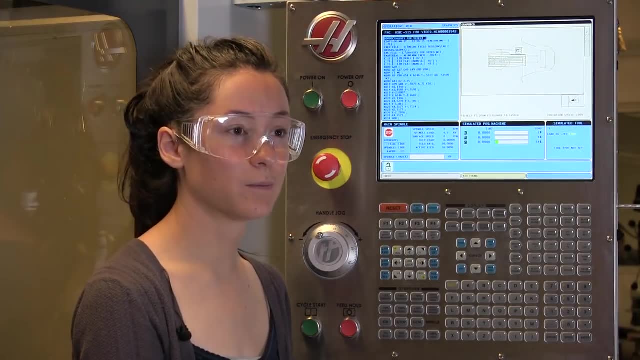 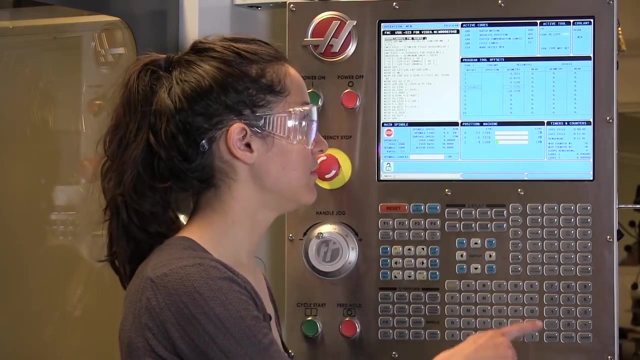 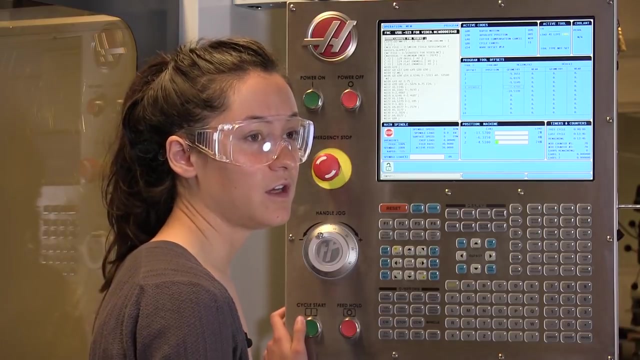 If everything looks correct on your program, then you're ready to start running it. To do that, you're going to press this memory button here. That will get you in the correct mode to run the program And then you're going to press the green button to start it. 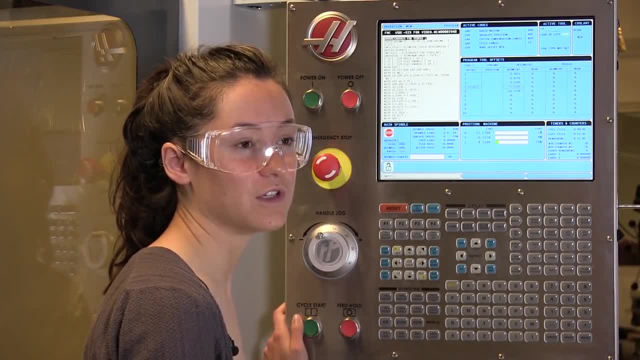 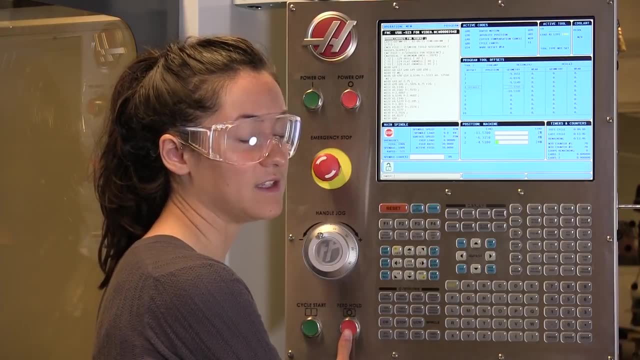 You'll press the green button after it changes tools and waits for you to confirm, And then you're going to want to make sure your thumb is ready over this feed hold button in case for some reason, it does a toolpath that doesn't look correct. 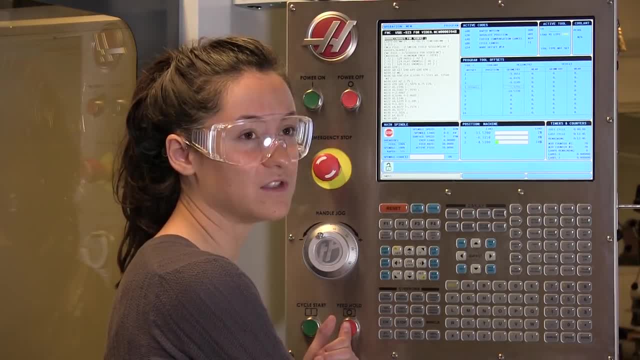 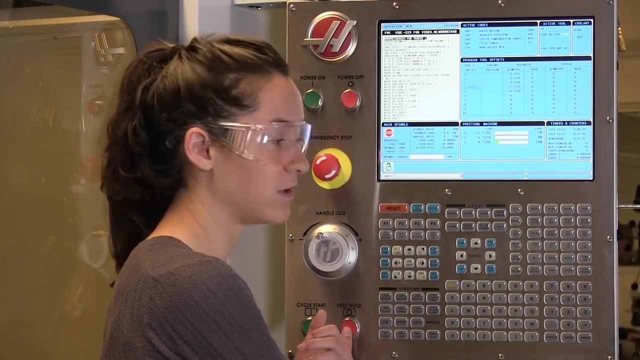 You could stop it. If it's heading towards the vice, you can stop it. If it's going through one of your mounting screws, go ahead and stop it. If you wanted to clear chips off the part or see what was going on, go ahead and stop. 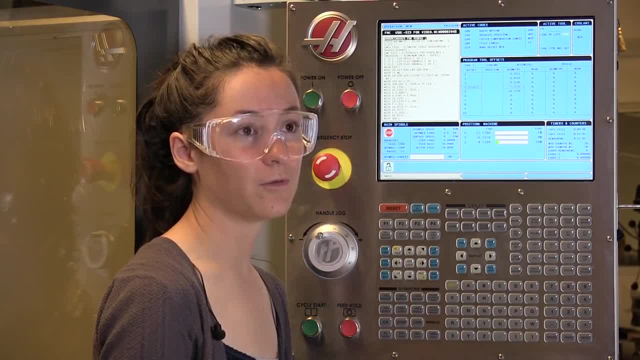 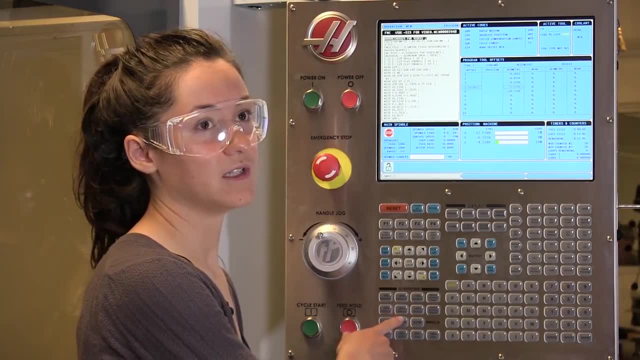 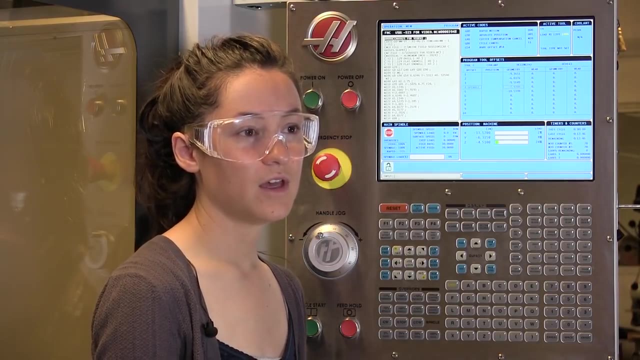 this button here. That'll just stop the table and spindle from moving around. The spindle will still be spinning, So it won't let you open the door unless you stop to stop the spindle. It's no big deal to press this button. The green button will just start it right back up from where you left off. 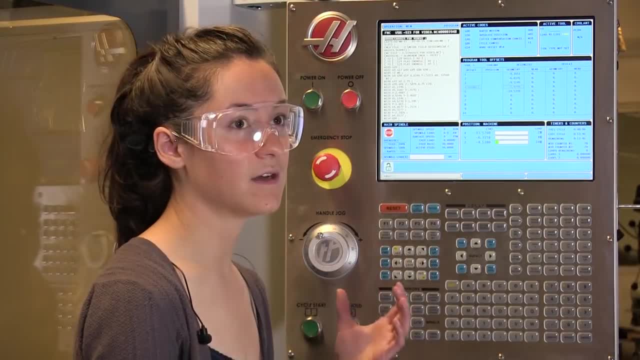 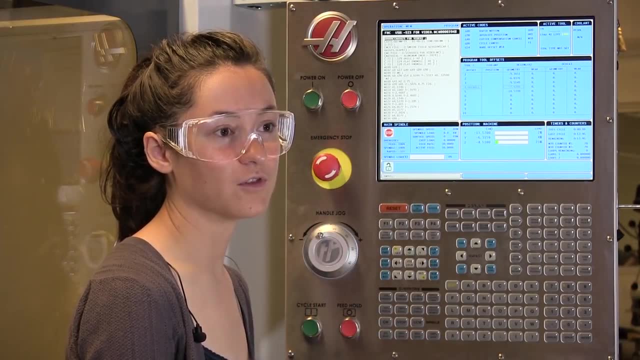 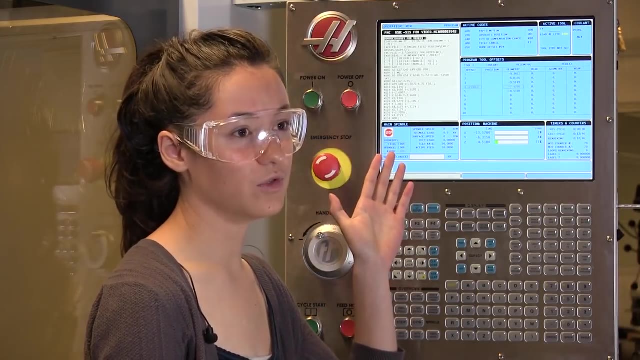 If, for some reason, the part gets pulled out of the vice and is stuck on the spindle, you're going to want to press the emergency stop button, Or for any other situation where you feel uncomfortable with what's happening. It's not easy or it's not possible to restart your program. 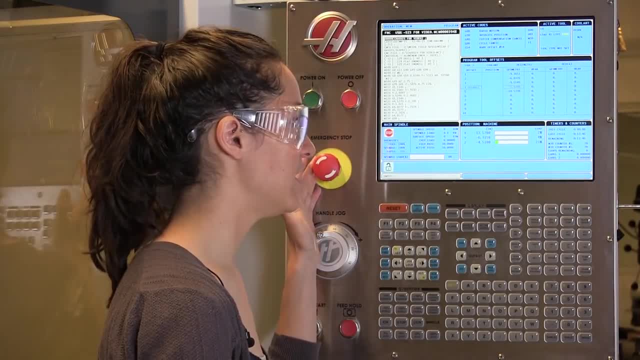 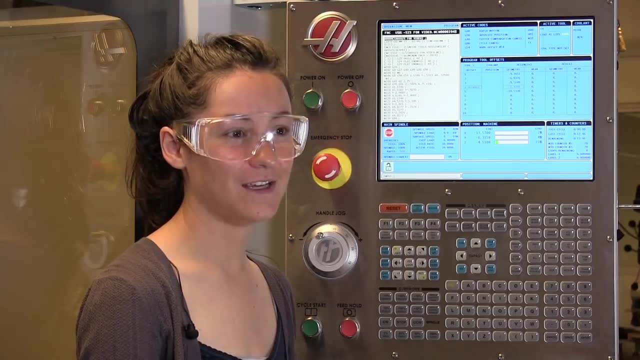 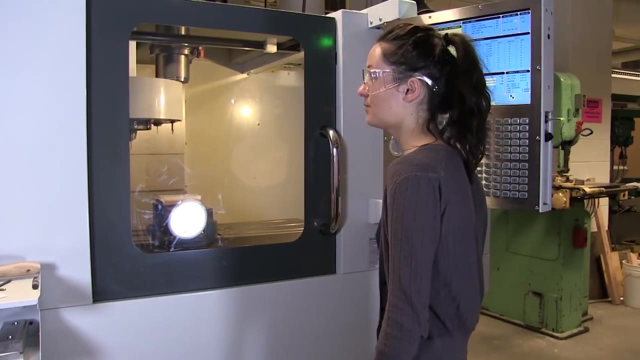 Restart your program in the middle if you press the emergency stop. So it's better to use feed hold, but always know that that button is there for you. So now it's ready to run the program, So just start green to start it up. 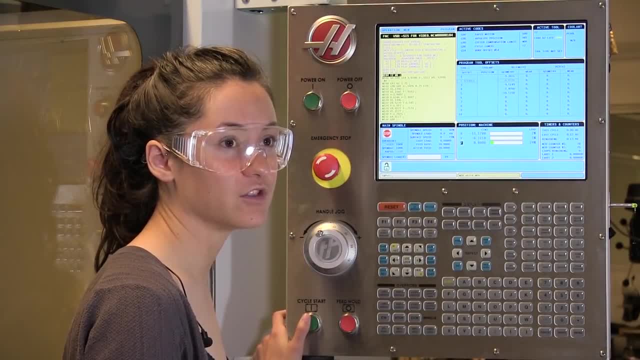 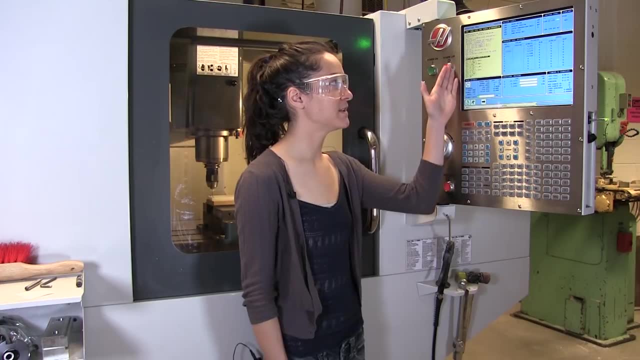 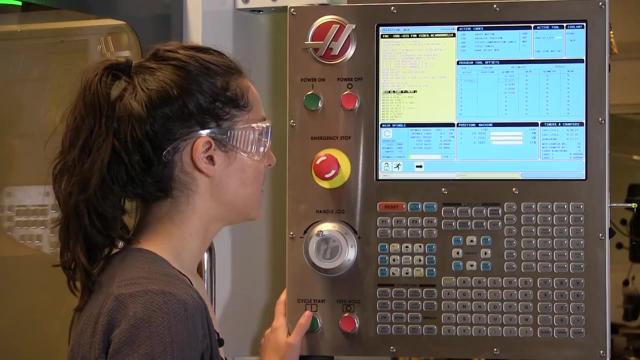 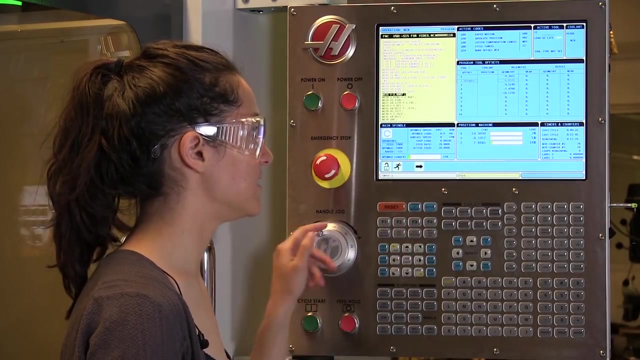 Now I'm going to push the green button because it changed tools into the first tool you're using Here. you can see it's stepping through your G-code. Also, pay attention to your spindle load here And this will report the feed rates and the spindle speed to you. 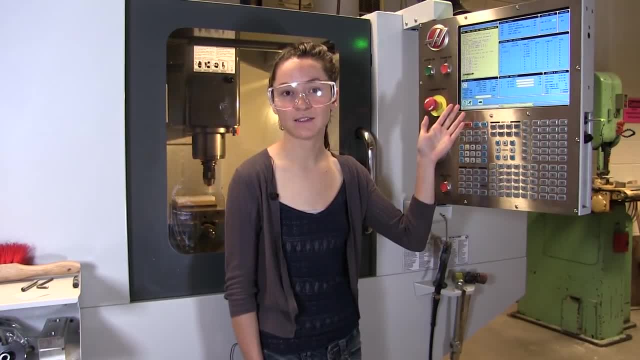 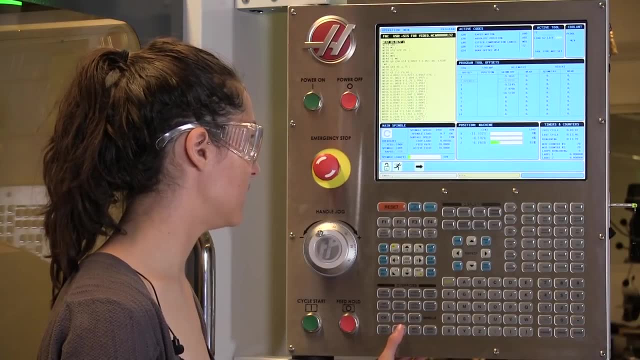 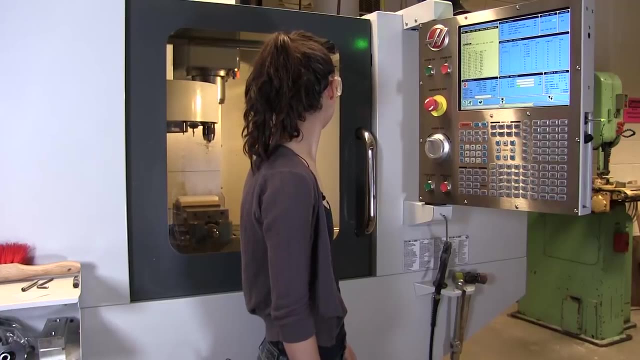 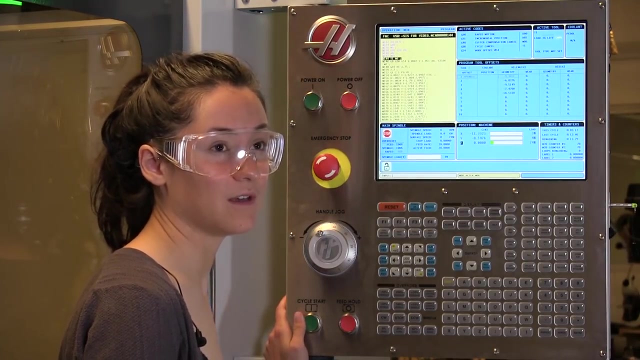 Rapid motion is set to 50% on this machine max, But if you feel uncomfortable with how fast it's moving between changes, you can step this down to 20%, To 25% or even to 5%. Now that it changed tools, it's waiting for me to confirm. 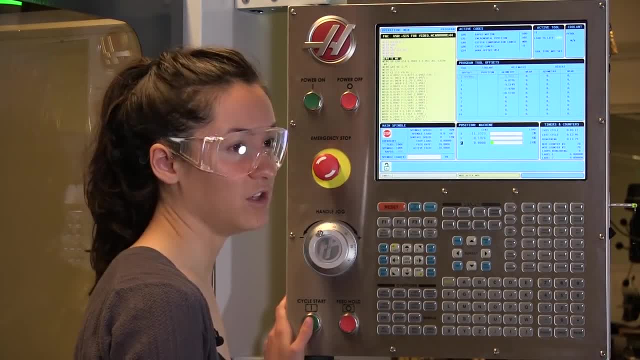 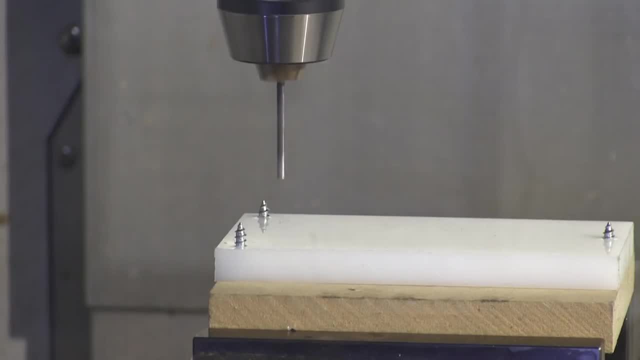 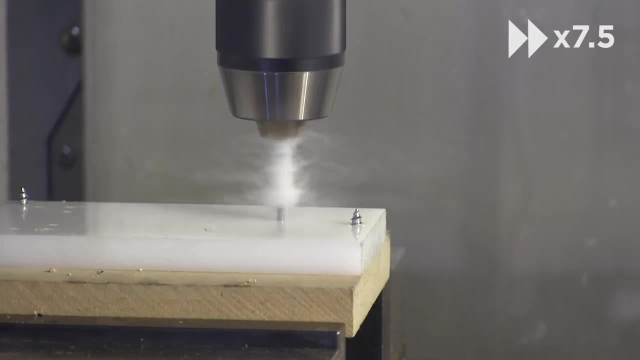 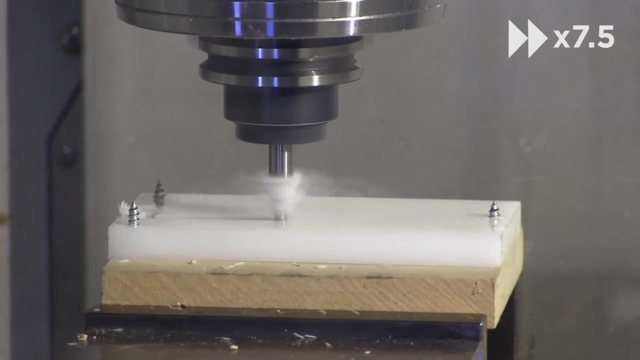 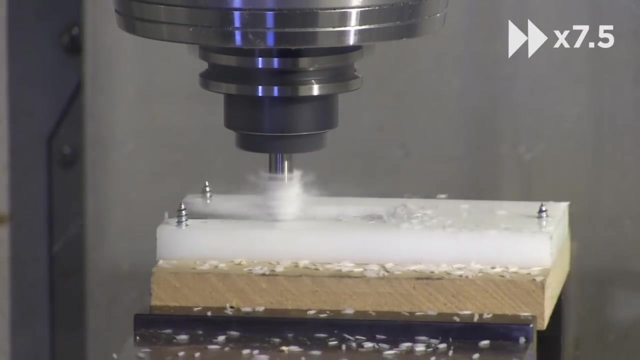 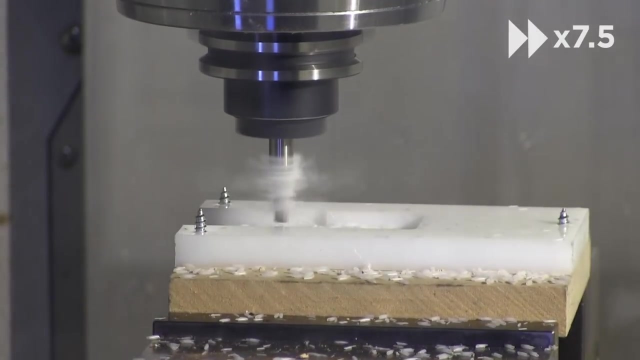 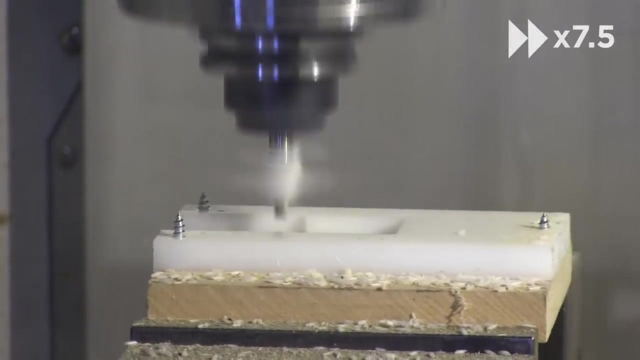 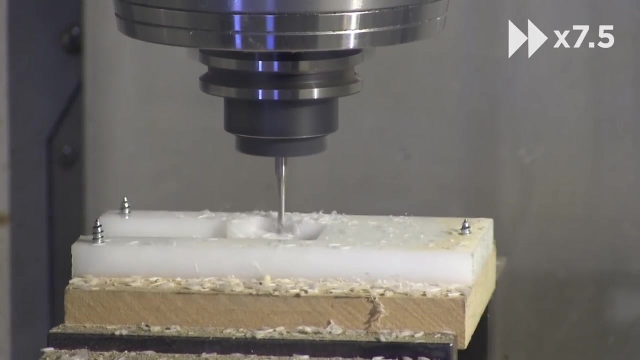 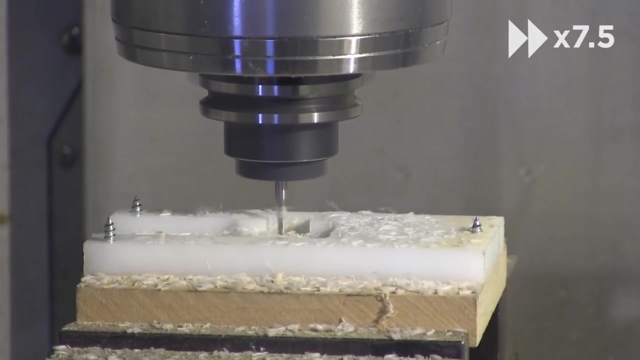 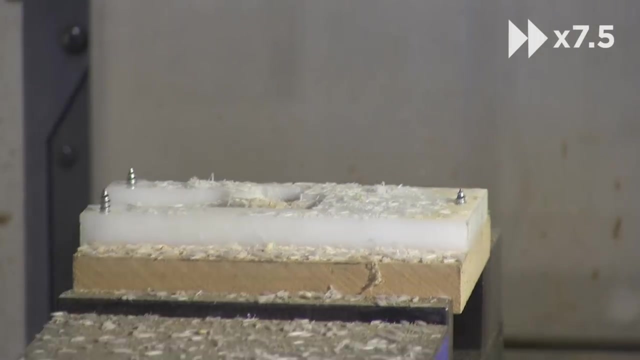 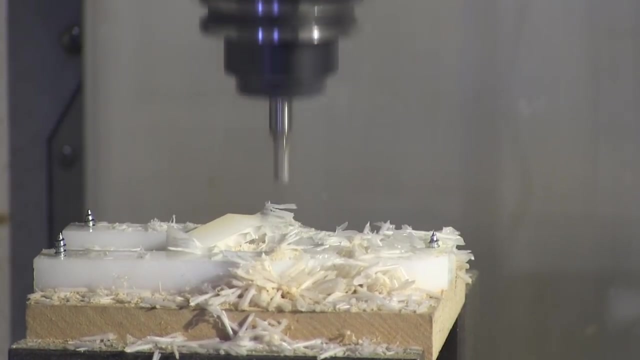 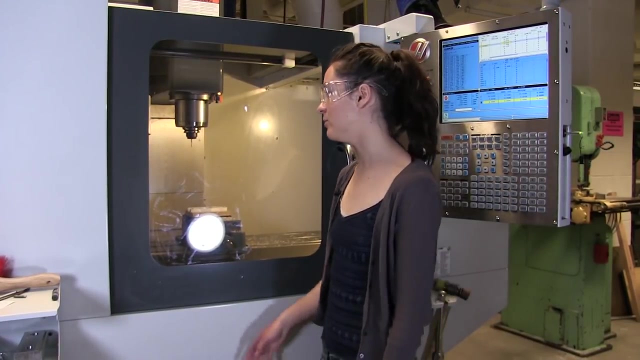 Also, this green light will be blinking. I'm just going to press the green button now to confirm that that's the correct tool. So I'm going to press the green button Now. I'm going to press the green button, Thank you. Now that your part is done, you're going to want to move it, so it's easy to get out of.